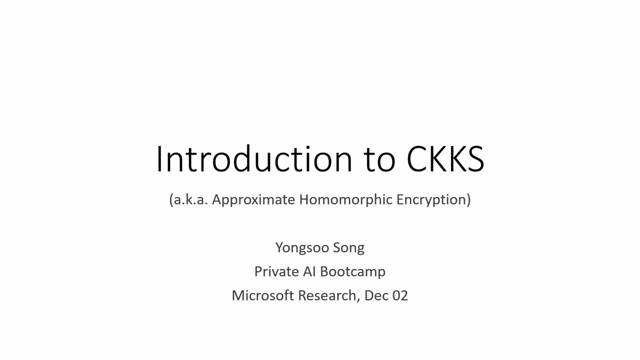 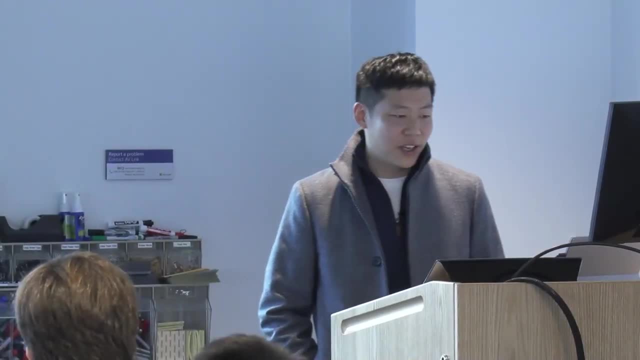 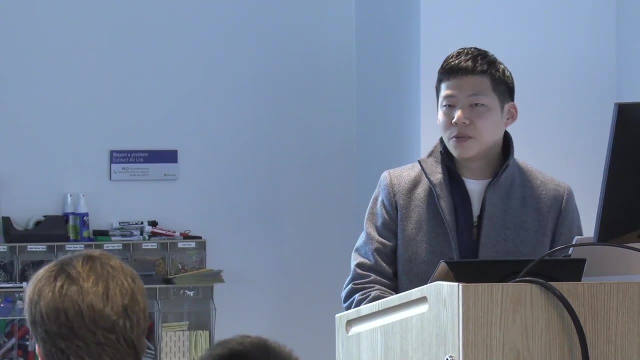 Thank you, Wei, for the introduction. Hi everyone, Good afternoon. I'll give a brief tutorial on CKKS, which is one of two homework encryption schemes supported by the Microsoft C library, And please feel free to interrupt if you have any questions any time. 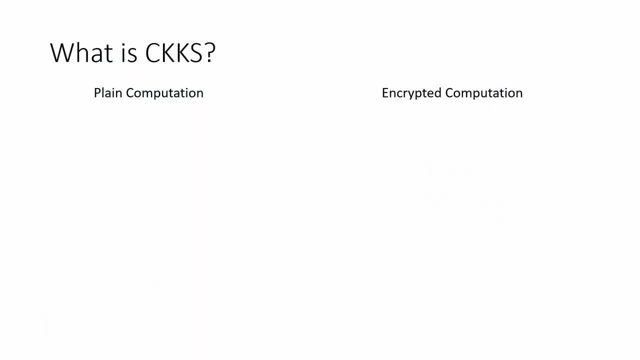 So ATA technology basically brings the plain computation to the encrypted world. So most of the homework encryption schemes, including BGV or BFV, support discrete computation as explained in previous session, such as Boolean arithmetic or integer arithmetic or modulo p operations. But in practice we also 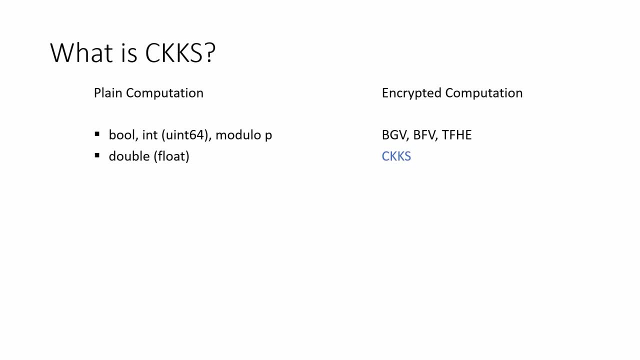 use some other variable types, such as double, to take some advantage of approximate computation, And the CKKS natively supports encrypted approximate arithmetic. Thank you. So basically, this scheme was designed in 2017.. And back then it was initially called. 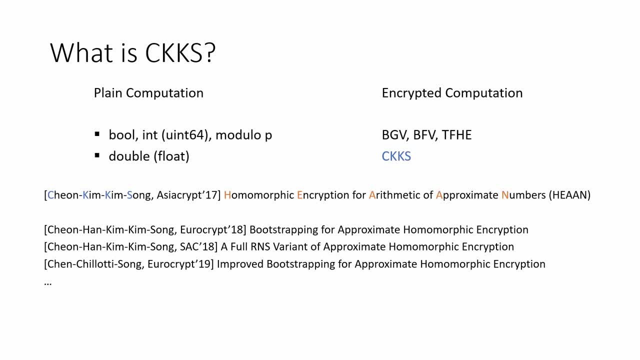 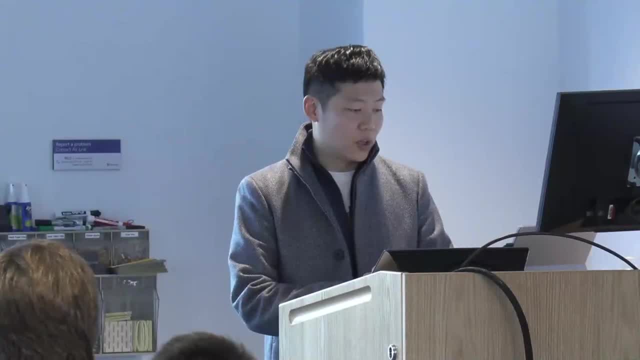 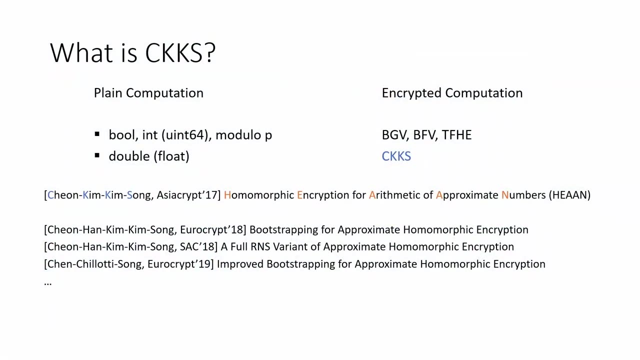 HEAN by the authors, But nowadays it is formally called CKKS after the author's name, to distinguish the name of this scheme from the name of public libraries which implemented the same scheme. So there has been a sequence of researches improving the functionality and efficiency. 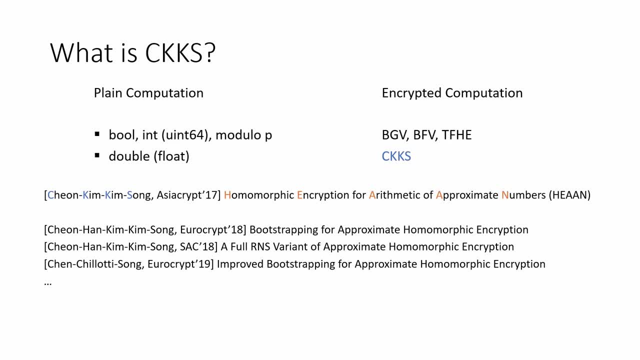 of this CKKS scheme And I give some high level idea about algorithms and API of C library in the CKKS mode so that you can play with it later without checking all the details of these papers. And the primary core of this talk would be to understand this example code in the C library. You can, if 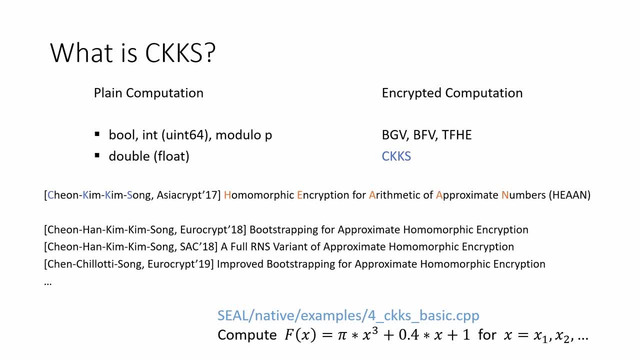 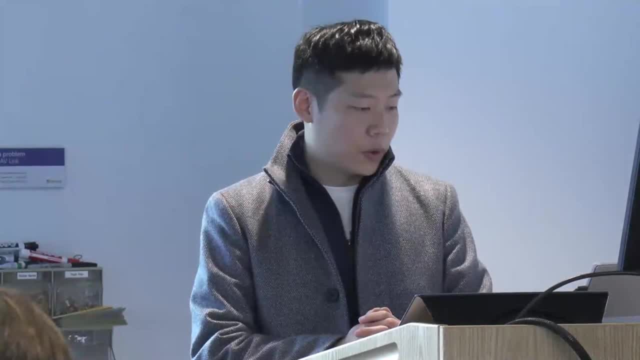 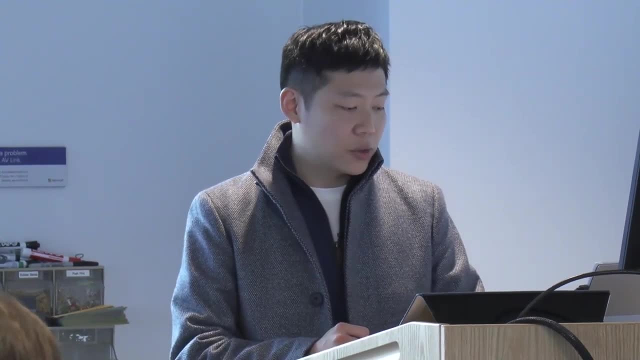 you have installed the C library, then you can just open this gpp file if you want. This code basically evaluate cubic polynomials and multiple real numbers, And another core is to learn some important concepts and languages widely used in H community so that we can 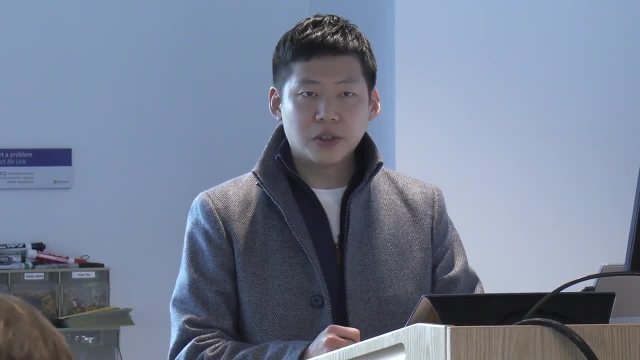 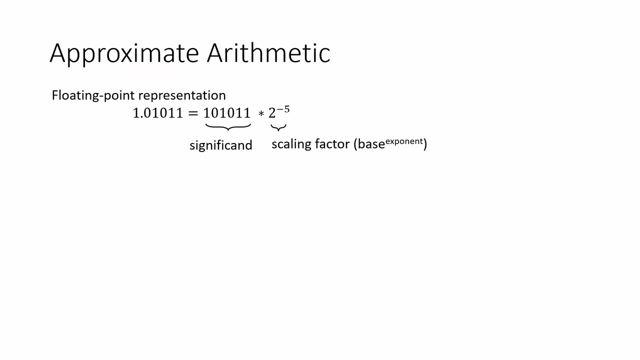 use these keyword during the boot camp discussions. So before we get started, let me first record the floating point and fixed point arithmetic, because it's sometimes confusing. So in the first attempt we can use this as ausa, but in the second attempt we don't. We have to use the code throughout the process. So we'll. 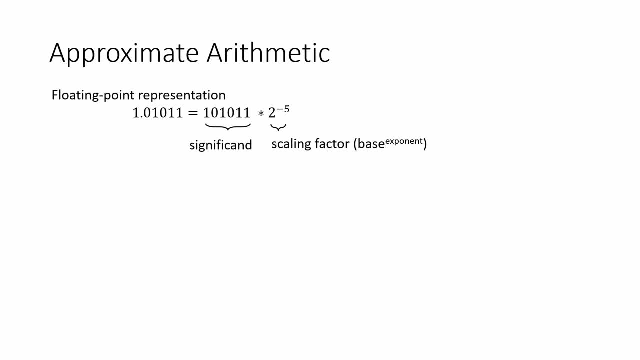 In the floating point number system, a real number is represented by a product of an integer called significant and a scaling factor which is usually represented as a base to the power of a base, And the intuition behind this representation is that the floating point number is not exactly the true value we want to store. 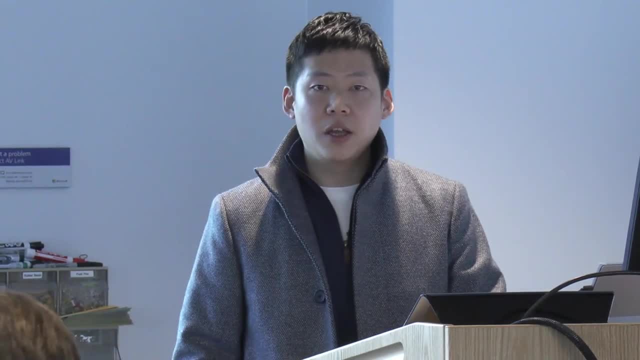 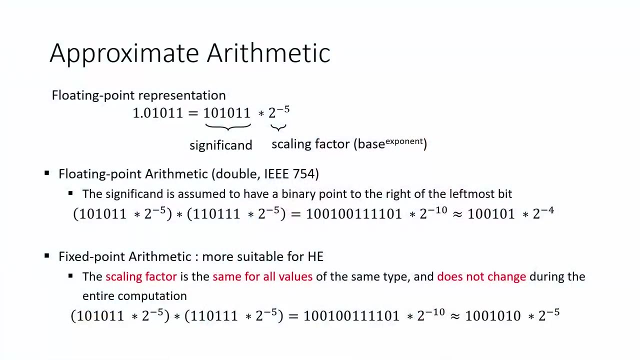 but it's just the approximate value which implicitly includes some numerical error after the radix point of the significant. And there are two, many method for multiplication between two floating point numbers. They are called floating point arithmetic and fixed point arithmetic. They are somewhat similar. 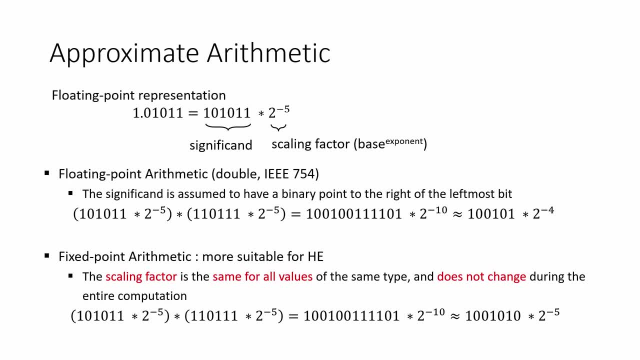 but both of them first multiply two significant bits and perform some rounding operation to make trade-off between precision and efficiency. But the main difference is that in the case of floating point arithmetic we always store a fixed number of bits of significant and scaling factor can dynamically change. 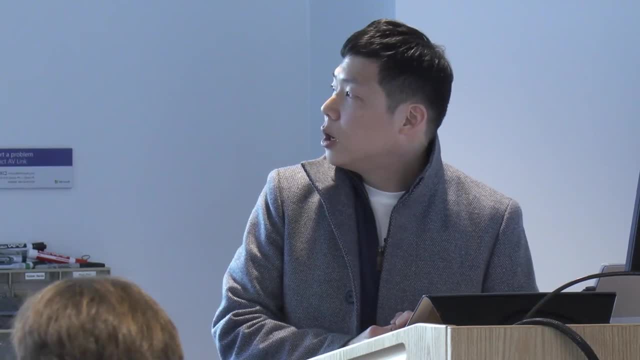 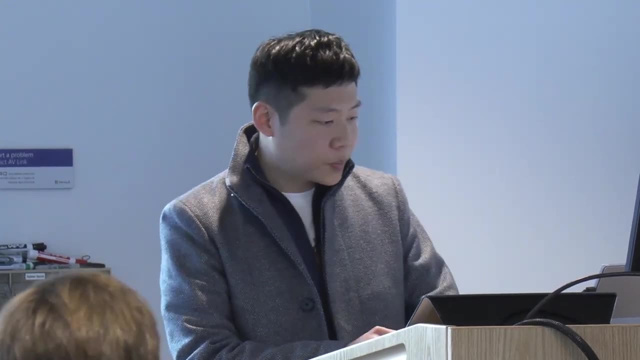 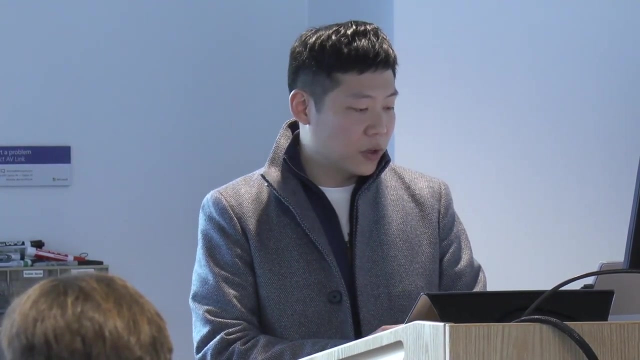 during the computation. As you see in this example our floating point numbers have six bits of significant. But in the case of fixed point arithmetic we keep the same scaling factor so that the bit size of significant may change. Here the inputs have six bits. 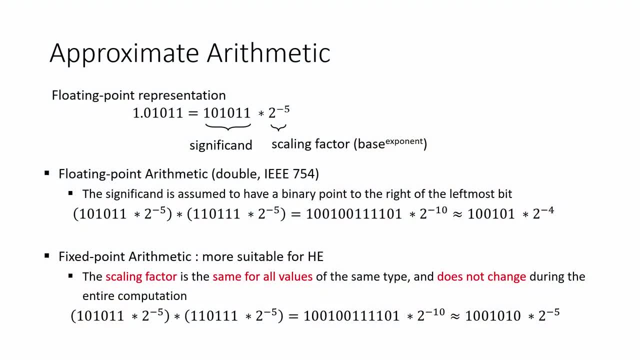 but the output significance is seven bits integer, But scaling factor is stable as two to the five. So in the case of encrypted computation the fixed point arithmetic is more stable, since we are now able to check the bit size of intermediate values during the computation. 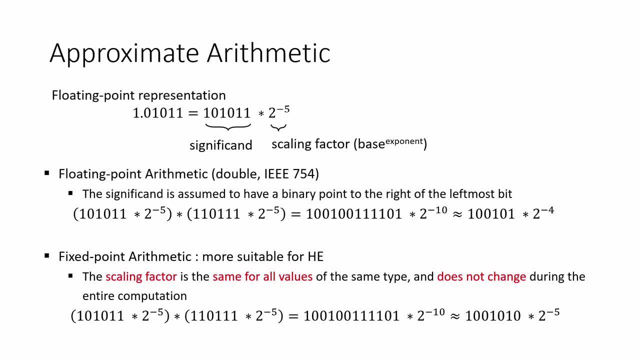 So in the case of encrypted computation the fixed point arithmetic is more stable, since we are now able to check the bit size of intermediate values during the computation. So floating point arithmetic is much more tricky. So, roughly speaking, scale case supports a sort of fixed point arithmetic. 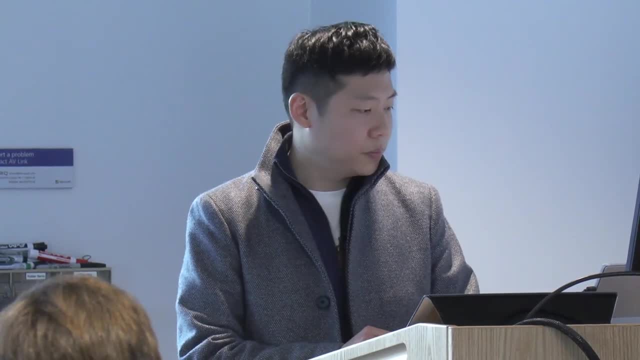 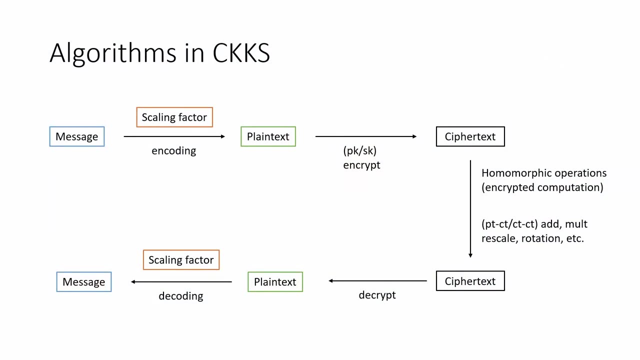 but with some extra noise from the system. So in this talk, methods and plaintext will refer to two different variable types. So methods should be a vector of floating point numbers or a vector of complex numbers, And it should be first transformed into a plaintext. 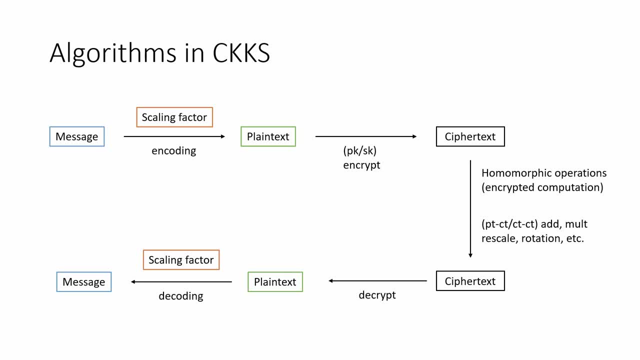 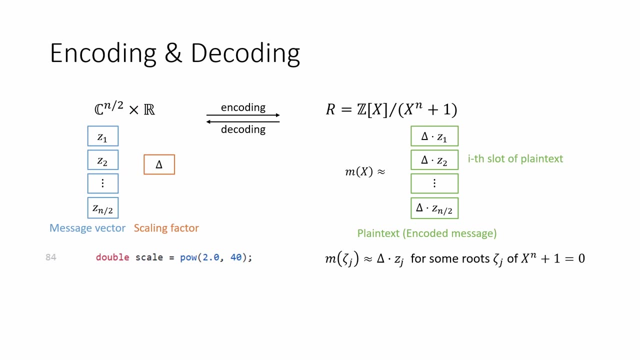 via a public encoding map before being encrypted, And the CKK scheme provides various homomorphic operations such as addition, multiplication, rescale, rotation. Encoding and decoding are public transformation between message and plaintext. As noted in previous session, the scheme works over the set of a polynomial modular x. 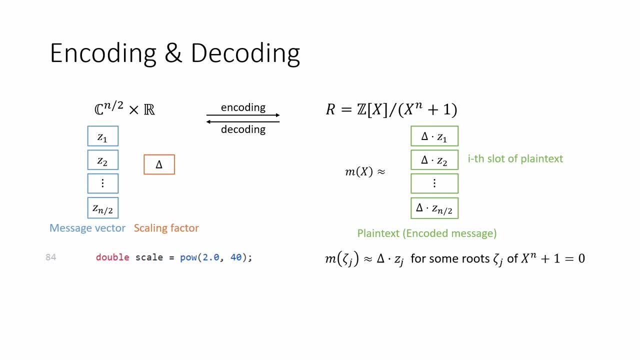 to the n plus 1.. The set is denoted by r And for a given message, which is a vector of n over 2 complex numbers, we first multiply it by a scaling factor and pack these n over 2 numbers into a single integral. 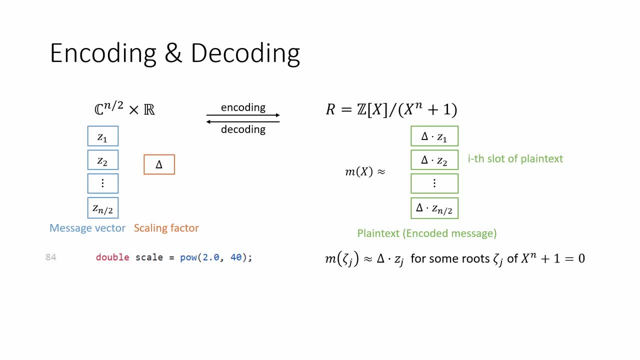 polynomial using some Lagrangian interpolation over this ring. You don't have to know all the details, but as a toy example, if you encode this pair of complex numbers with scaling factor 2 to the 7, then we use this. You end up with this integral polynomial m. 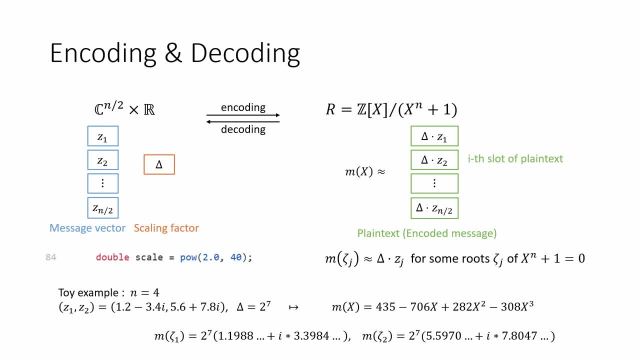 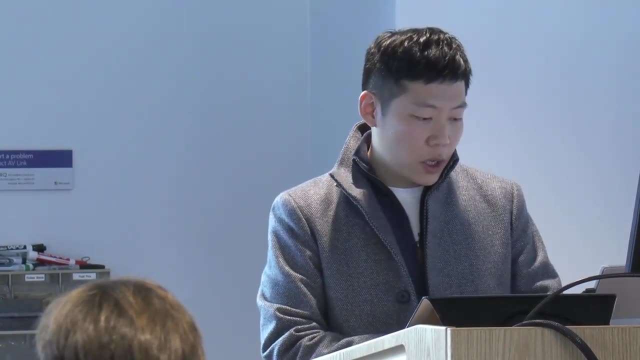 And we can double check that. if you evaluate two roots of unity at m then you recover a kind of approximate values of 2 to the 7 times of the input vectors, And later CKK's scheme will support some parallel computation on these multiple slots. 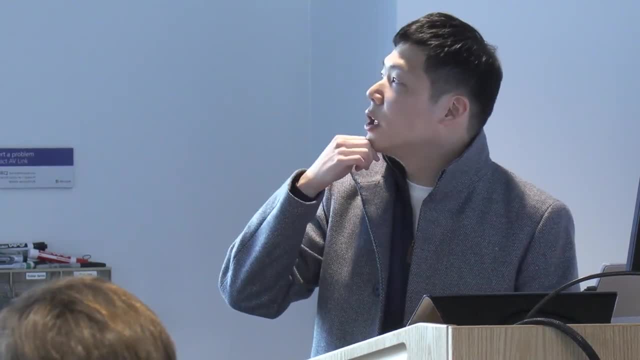 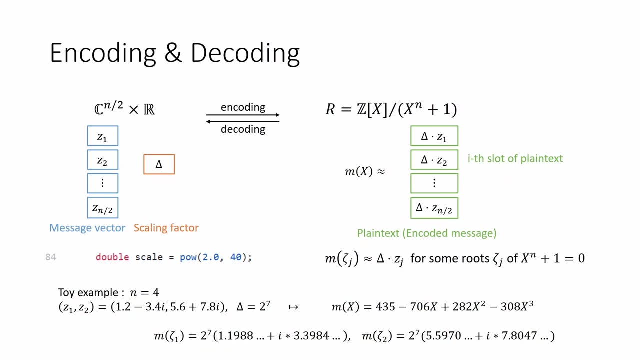 This individual. So you can imagine that a plaintext implicitly has some n over 2 plaintext slots. Each of them can store a complex number And, after encoding, each of these slots contains some approximate values of delta, times zi, And you should use a larger data to keep more precision. 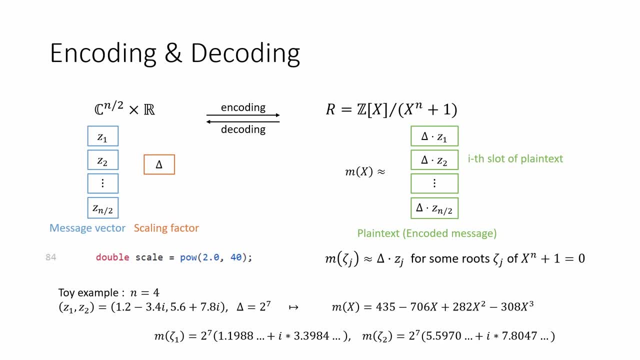 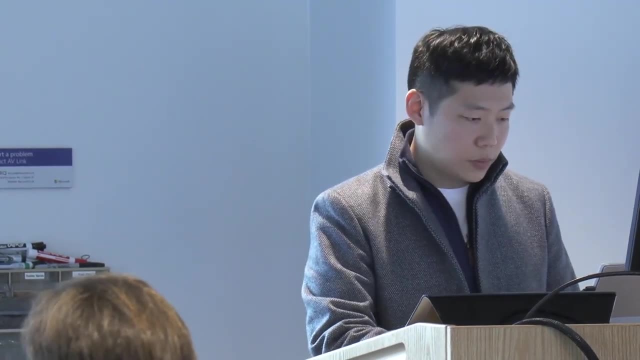 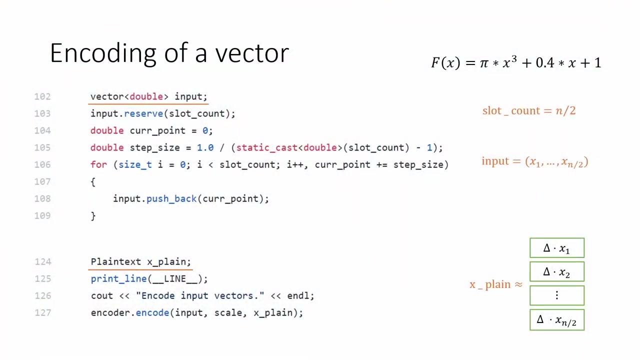 because m is basically an integral polynomial. So this encoding algorithm includes some randomness. So if you use two small scaling factors then you lose too much precision significantly. after red X point: OK. So in the source code we first initialize the imp factor. 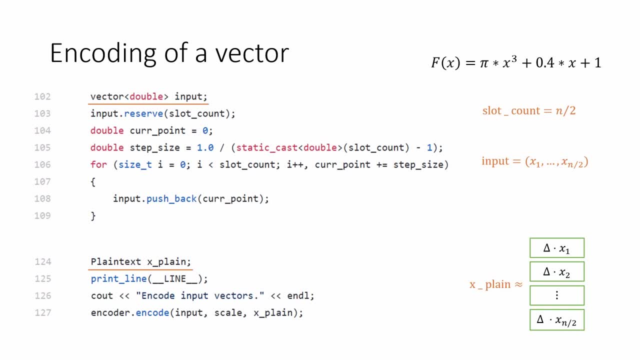 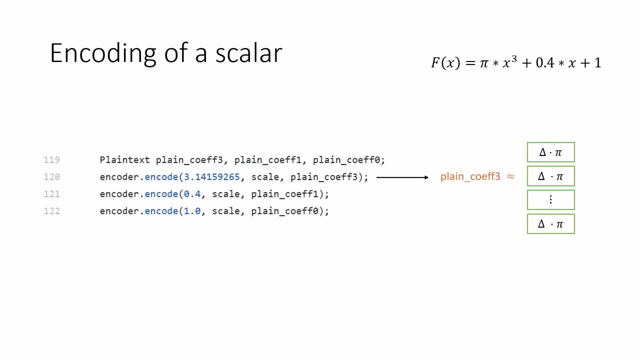 which is n over 2 dimensional vector of real numbers between 0 and 1, and use the encode function to encode it into a plaintext. Let's see what the plaintext explains. And we are going to evaluate this cubic polynomial, So we should also encode the coefficient of this polynomial. 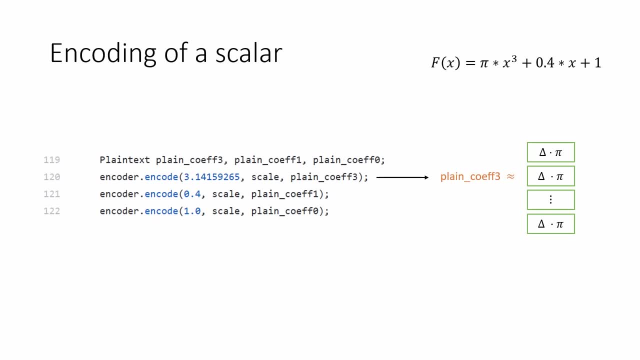 as well. They are pi and 0.4 and 1.. It's simply a scalar. So if you encode a pi, then it is mapped to a plaintext which contains delta times, pi in order. So this is a plaintext. This is a plaintext. 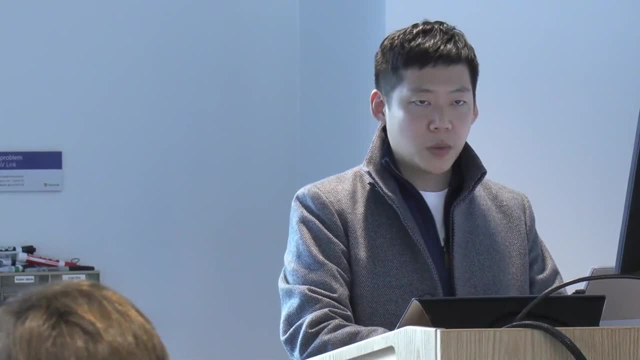 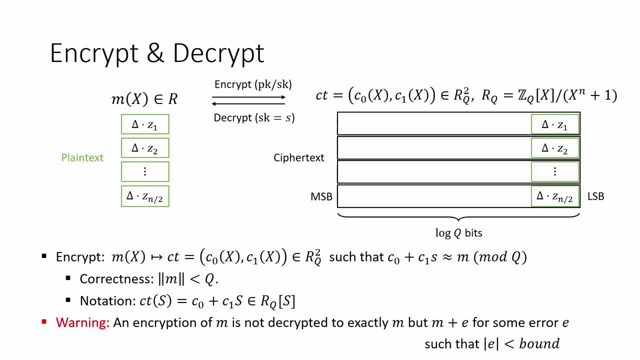 OK, So R sub Q denotes the residue ring of R modulo Q, which is the set of integers, set of integral polynomial modulo X to the n plus 1, with coefficient in Z modulo Q. So the secret key of CK case is a polynomial S And um. 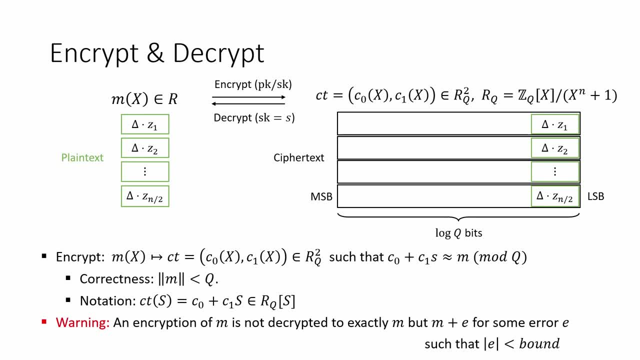 public key or symmetric key encryption over plaintext. M is a pair of polynomial C0 and C1, such that C0 plus C1S is approximately equal to M modulo Q. So it means that this C0 plus C1S modulo Q is the decryption circuit of CK case system. 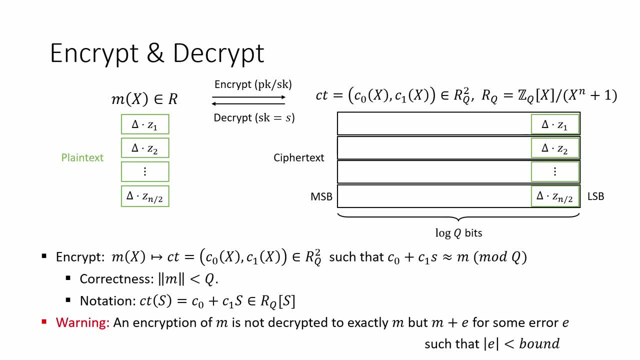 so that the decryption circuit correctly recovers the plaintext M if M is smaller than Q. So that's the problem, OK, OK, Otherwise we will have some modulo Q reduction in M and the result would be incorrect. So for simplicity we often write the ciphertext CT. 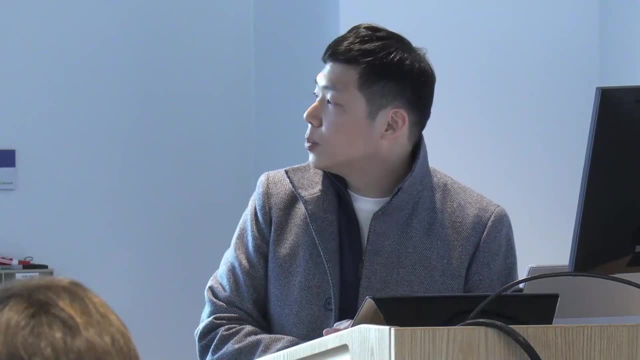 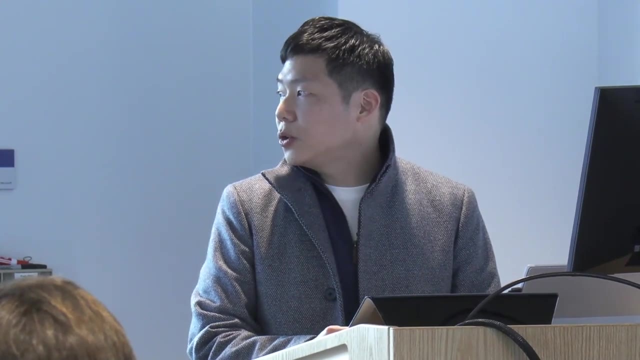 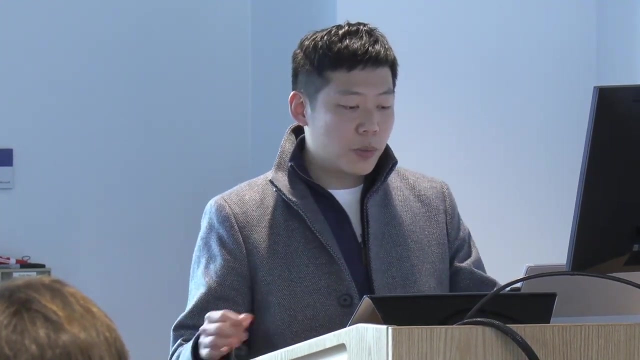 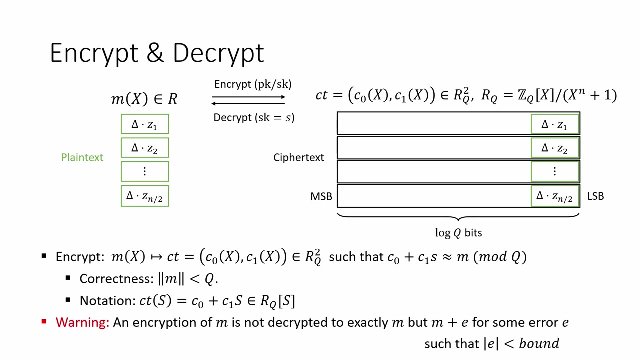 as a linear polynomial C0 plus C1S And decryption circuit is just a sub-shifting S by the secret key, small s. So you can just imagine that You store plaintext blocks N over 2 plaintext blocks in larger black boxes of size roughly logo qubits. 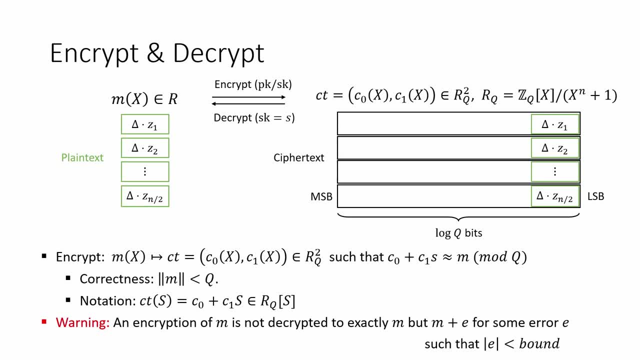 And only SK secret key owner can open this black box. And the size of this black box is represent parameterized by this important parameter Q. And remember that this encryption algorithm introduced some small noise to ensure the security, The security of AC system. So the C0 plus C1S is not exactly equal to M. 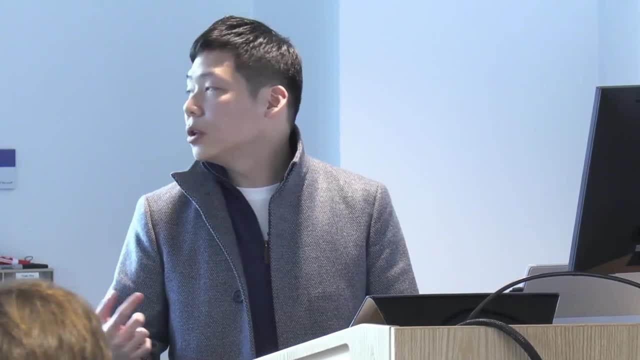 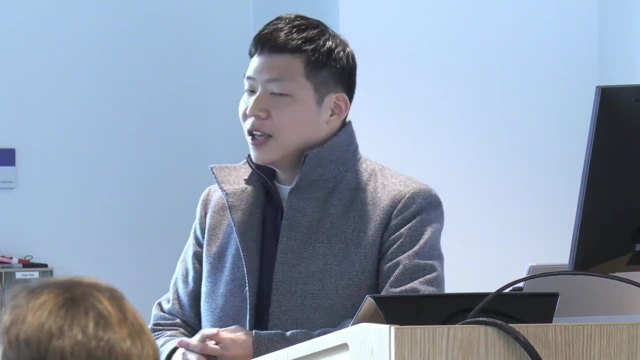 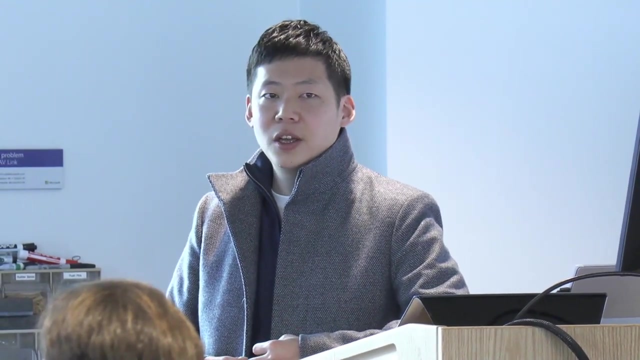 but it's just approximately equal to M. So the noise different from the BFV scheme explained in the previous session. in the case of CK case we don't distinguish noise from plaintext. Noise is considered as a part of message, It is just considered to be a numerical error. 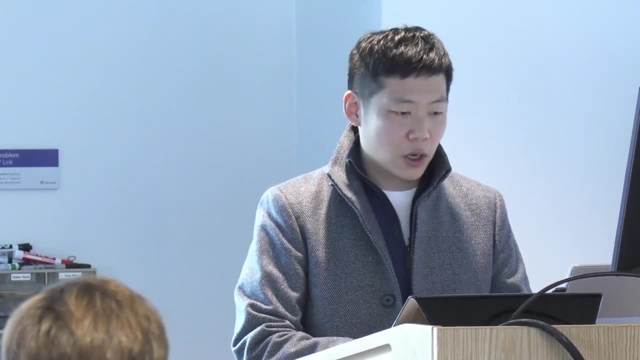 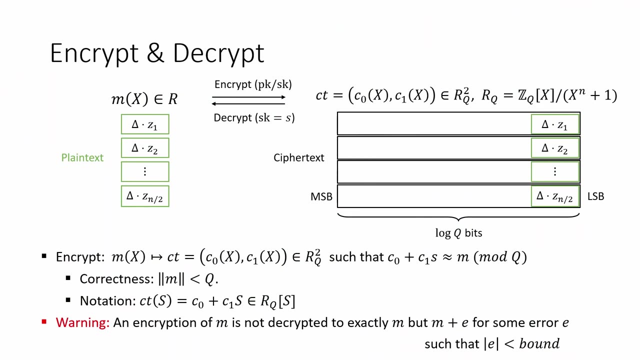 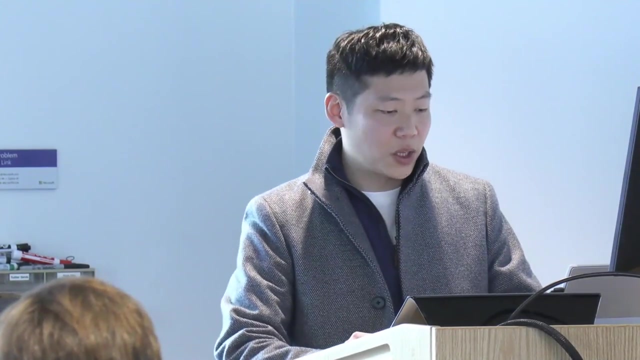 during approximate computation. We anyway work on it. We work on approximate numbers, with some error. So if you encrypt 0 and directly decrypt it, then you don't get 0, but just a very small number which has no upper bound depending on the parameter of AC system. 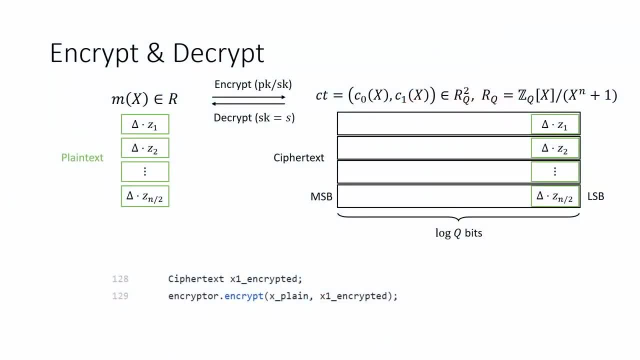 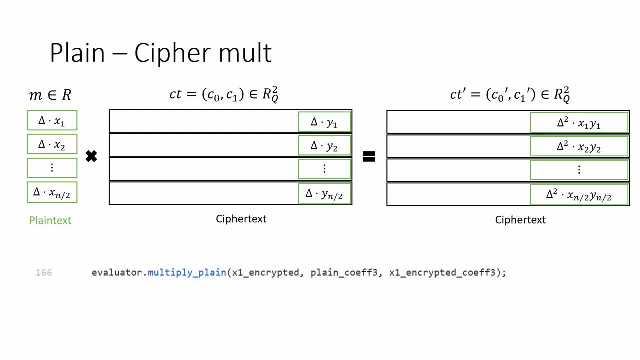 And encryption function is in the line 129 in the source code, And the CK case scheme supports addition and multiplication between plaintext and cyphertext or cyphertext and cyphertext. First of all, the multiplication between plain and cypher returns the cyphertext of the same black box size, which 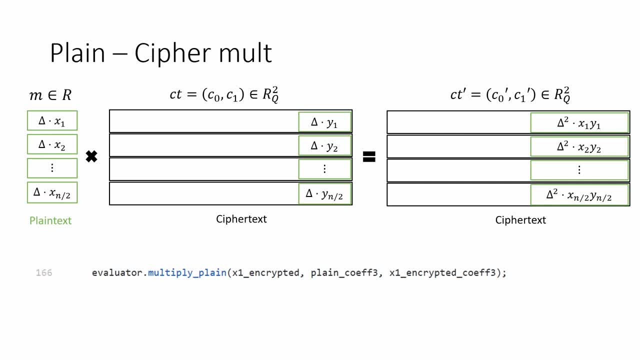 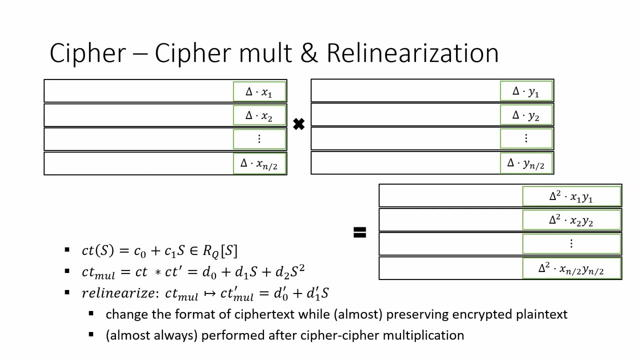 includes the product of this green plaintext blocks inside of it, So you can just compute the multiplication between plaintext inside of this black box And in the case of cyphertext multiplication. it's very similar to the previous case, but a bit more complicated. 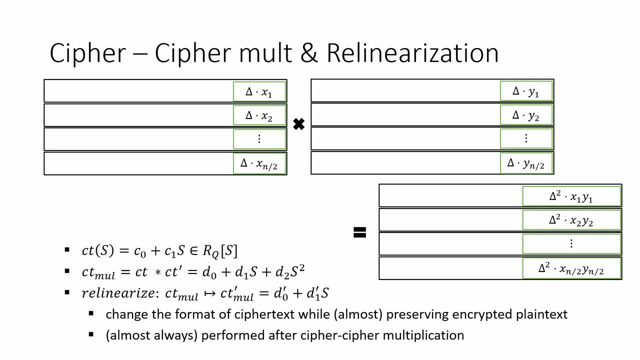 Because if you multiply two cyphertexts then you get the same size black box which includes encrypted product of two plaintexts And record that the plaintext or cyphertext is usually written as a dislinear polynomial, So technically you just simply multiply. 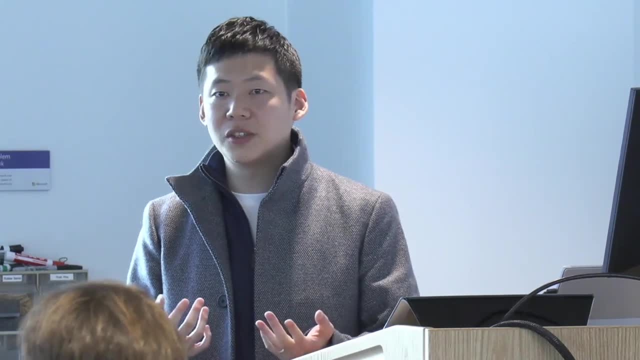 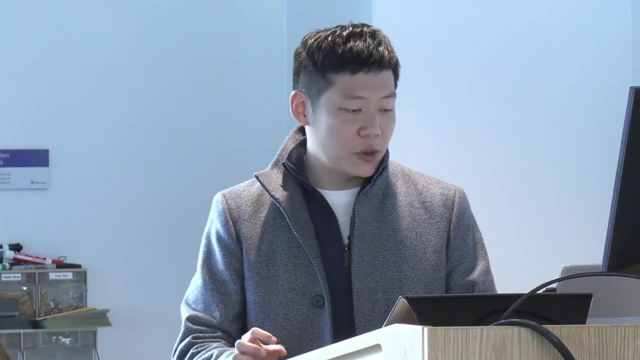 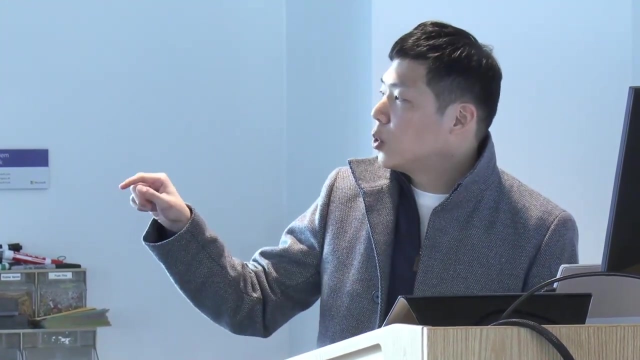 two cyphertexts and returns a quadratic polynomial because it's a product of two linear polynomials. So this homomorphic multiplication is usually followed by another operation called re-linearization, which transforms this quadratic cyphertext back to the linear cyphertext. 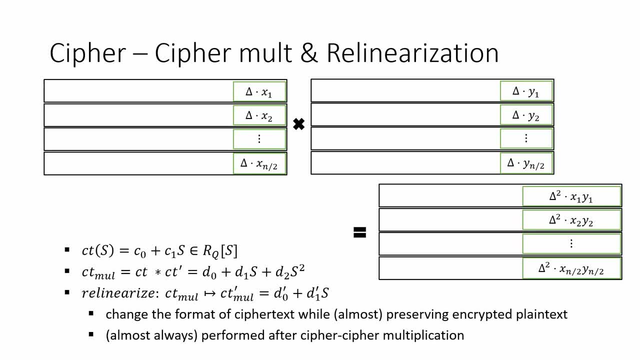 while almost preserving the encrypted plaintext. So, roughly speaking, if you perform the composition of homomorphic multiplication and re-linearization, then it will return a linear cyphertext which encrypts the product of plaintext blocks of the two input cyphertexts. 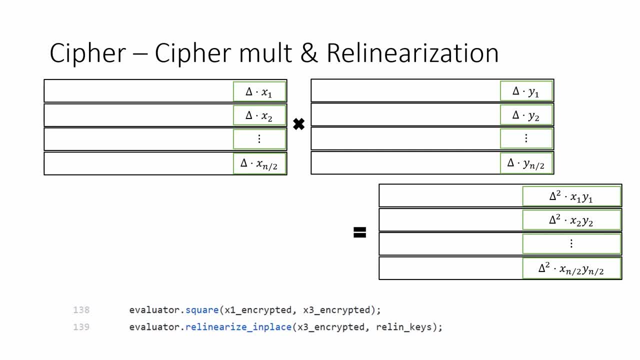 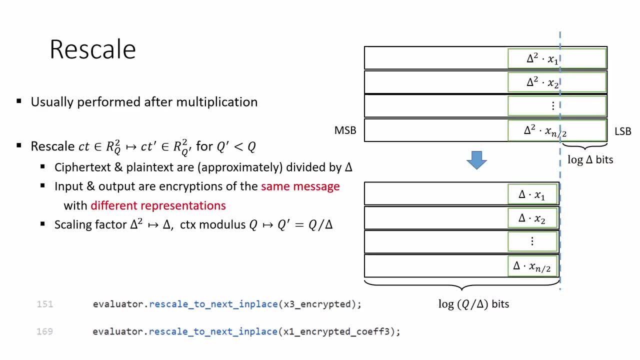 So this is the source code And this procedure requires some extra public parameter called the linearization key. So re-scaling is the key operation which makes CKCAS have its own characteristic and benefit. So this re-scaling operation works just like the rounding operation of fixed point arithmetic. 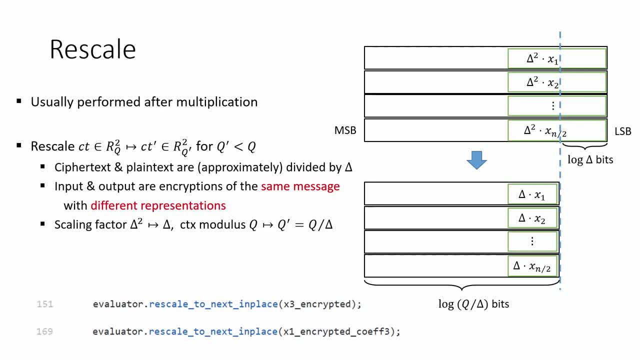 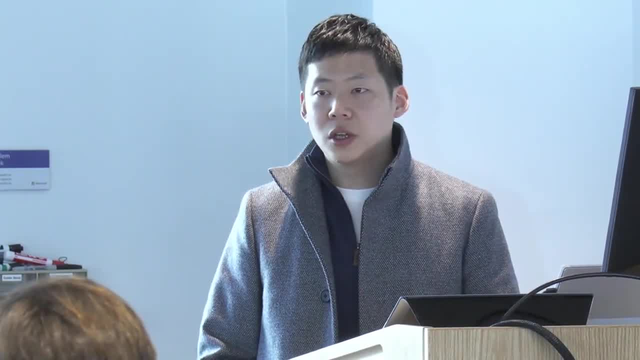 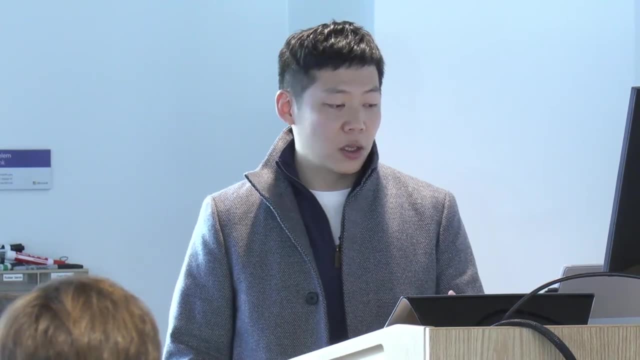 So after homomorphic multiplication the scaling factor over an encrypted plaintext becomes delta squared from delta. So if we repeat homomorphic multiplication then the scaling factor will grow exponentially as the computation progresses and the plaintext will overflow the size of this black box very quickly. 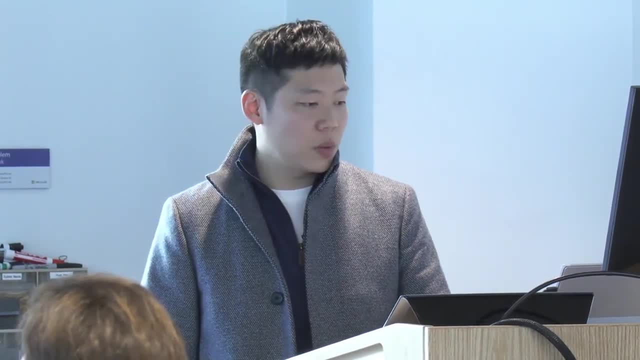 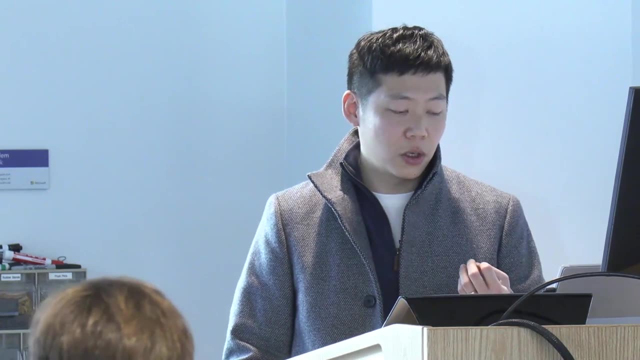 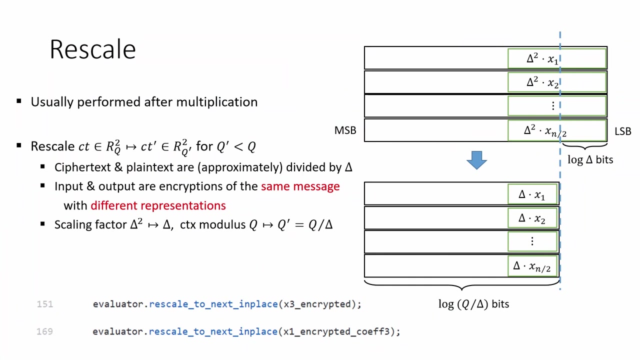 So, similar to the case of fixed point arithmetic, the re-scaling operation divided the cyphertext by data and cut off the least significant bits. log delta of cyphertext module TOI and thereby plaintext. So we recover the scaling factor. 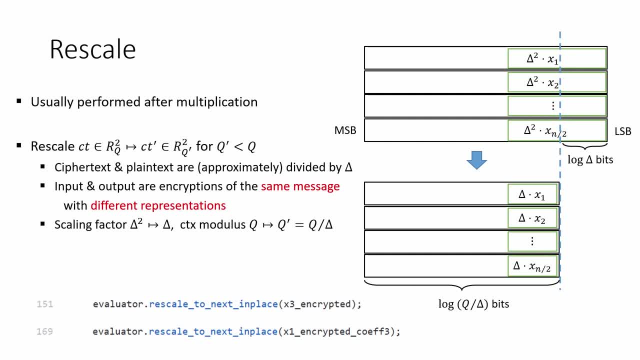 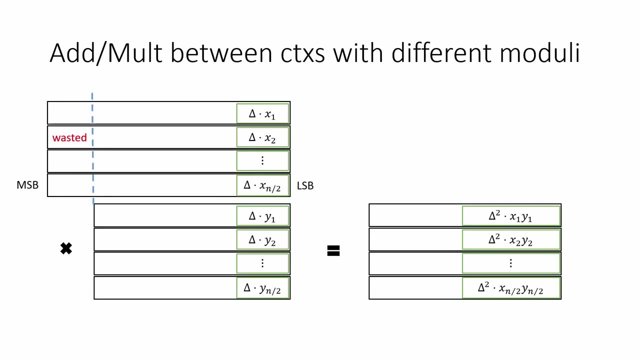 Yeah, delta after rescaling procedure. This is why the rescaling procedure usually comes after homomorphic multiplication, to maintain the same scaling factor during the computation. So the ciphertext modulus can decrease during the computation by rescaling. but what would happen if we multiply two ciphertexts with different moduli? In this case there's no. 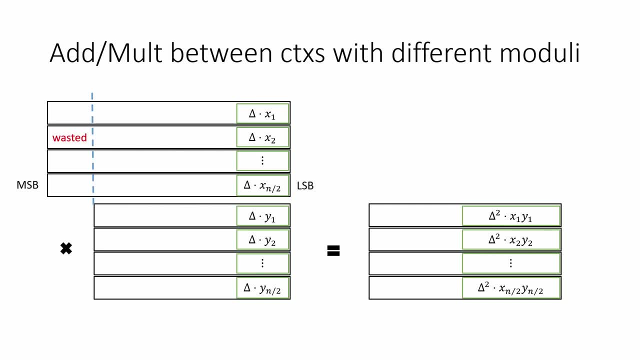 good solution of multiplying two, but we just have to discard some most significant bits of a ciphertext with your larger modulus so that we make them have same ciphertext modulus before performing homomorphic operation. So, as you can see, this is not an ideal situation, because we are not fully utilizing the computational capability of the ciphertext. 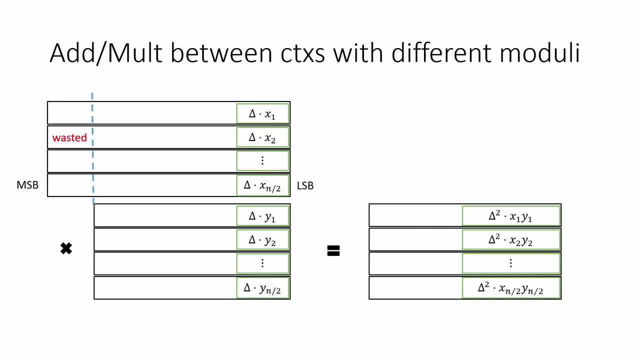 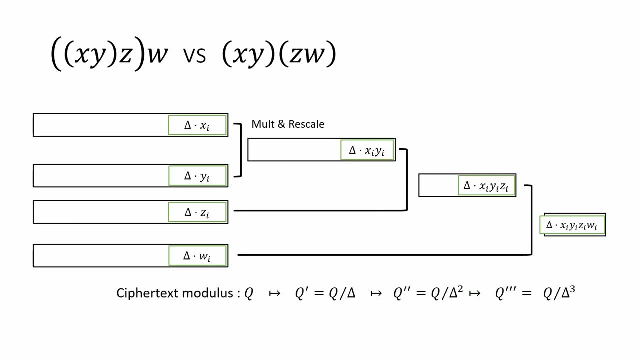 So it is very important to choose the best circuit representation without this unbalanced multiplication which basically wastes ciphertext modulus. So let's look at a simple example. We just want to compute the product of four ciphertexts. We can consider two different circuit representations of the same function. 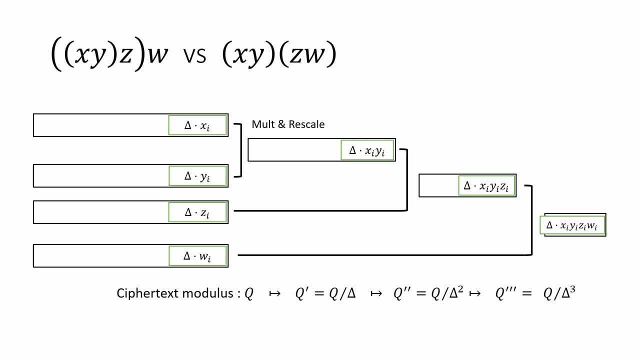 If we use the same function we can consider two different circuit representations of the same function. If we use the first representation, we basically have three multiplications, but two of them are unbalanced multiplications. So we consume log delta bit three times. So final ciphertext. 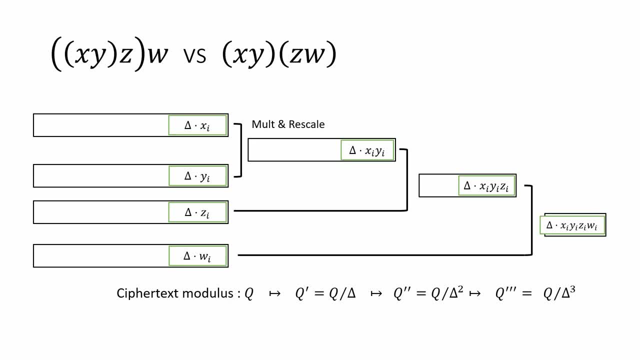 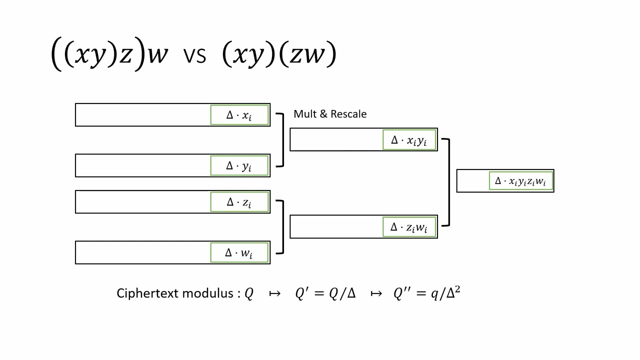 modulus would be Q divided by delta to the third. So as you can see in this figure, we could. the overflow could happen if this encrypted plaintext is larger than the size of this black box. But in other case, if we use this tree structure, then we finish the computation while consuming only two log delta bits of. 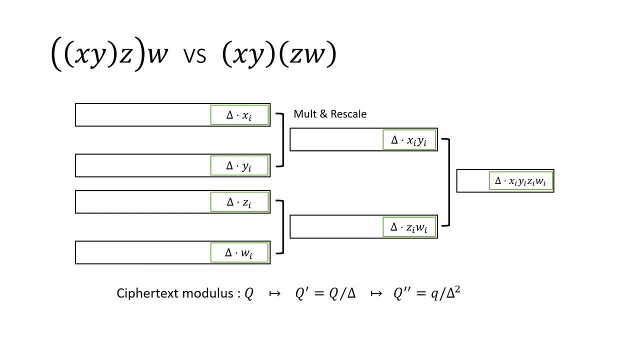 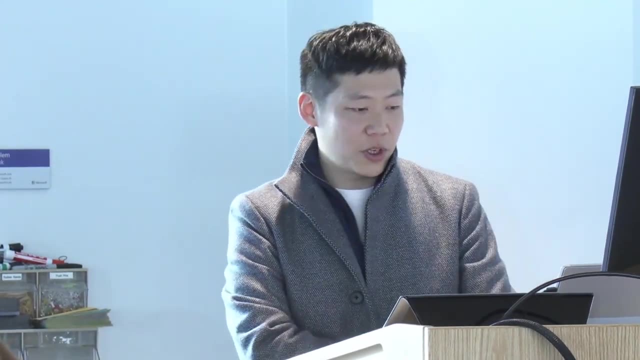 ciphertext modulus- And we are taking ciphertext- still has a large enough modulus for correct decryption. Okay, So I believe you probably got some intuition. Okay, So you probably got some intuition. So I believe you probably got some intuition why the depth of a circuit is so important. feature in HA. 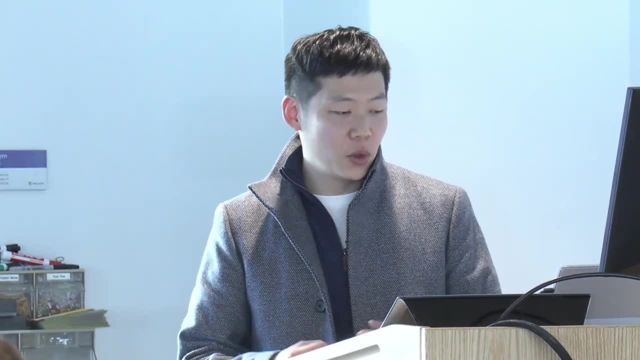 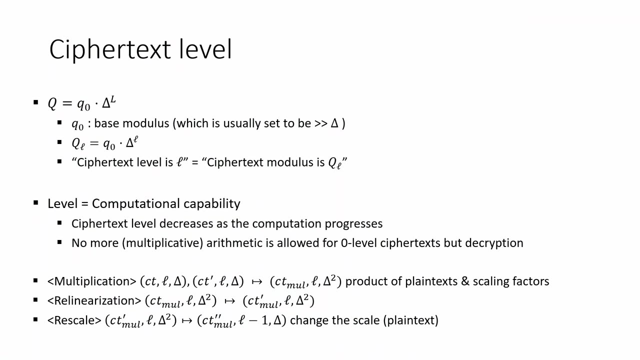 evaluation. So the HA community formalized this notion and we came up with some keywords like a level Ciphertext. modulus is a product of base, modulus Q0 and a power of base scaling vector delta, And we say that a ciphertext has a level L. 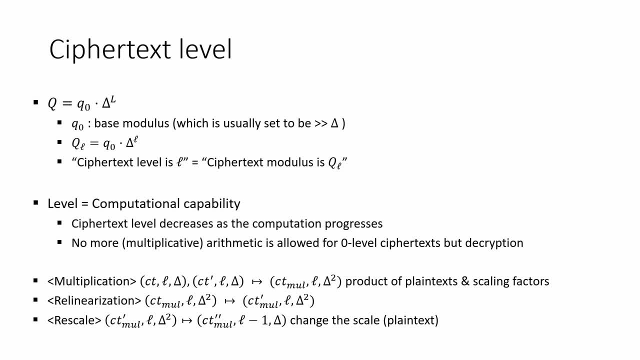 If its ciphertext is modulus, is Q sub L, which is a product of Q0 times delta to the power of L. So this level of ciphertext is a good indicator which effectively presents the computational capability of ciphertext. So if the level is decreased by one, 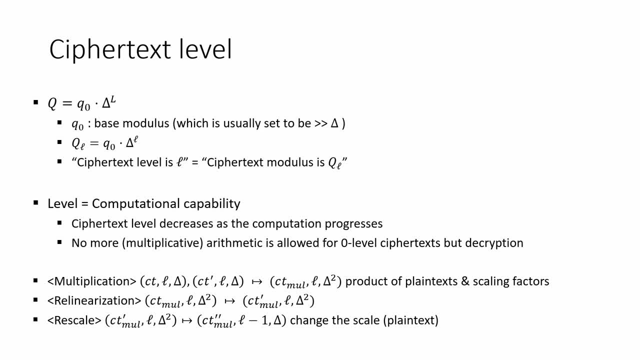 usually after Each of the multiplication, And we consume this all L level and no more arithmetic is allowed when a ciphertext reaches the lowest zero level. So no more multiplication is allowed for zero level ciphertext. So we can use this language to explain the functionality. 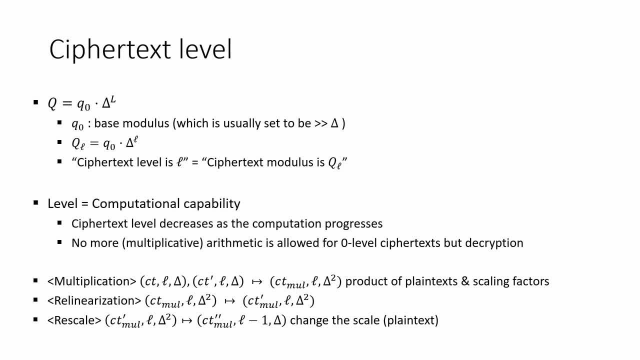 of CK-CAT algorithm easily. So a ciphertext is usually labeled with its level L and scaling vector delta, And you can see, You can check how homomorphic operations change this label information of ciphertext. So, for example, if you perform rescaling operation, 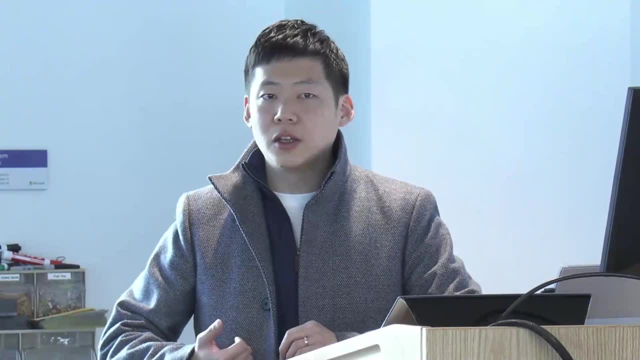 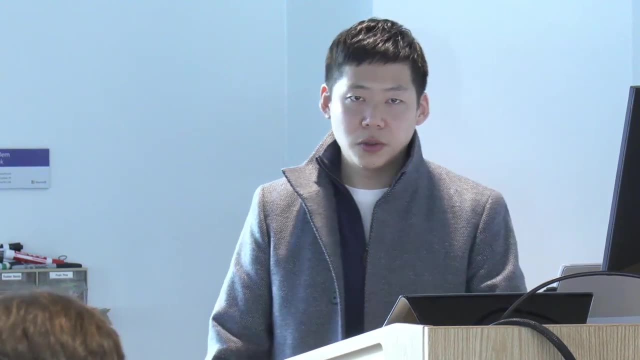 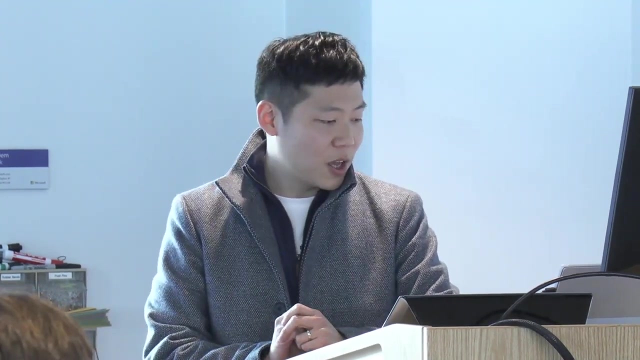 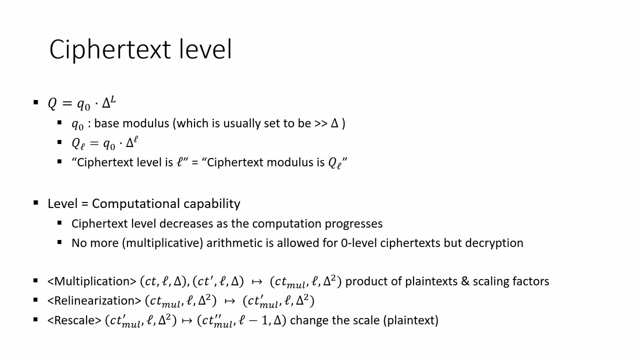 on ciphertext, then level is decreased by one And the scaling vector becomes to changes, to delta, from data square. And, as you can expect, the cost of encrypted computation heavily depends on the depth of homomorphic system, Homomorphic encryption system. So when you bring a computational task into an encrypted world, 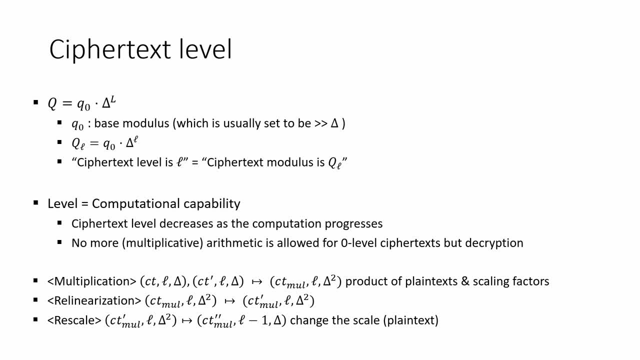 the overhead between displaying computation and encrypted computation is not a constant, But it heavily depends on the depth of circuit. So in general, an optimal algorithm in computational number theory may not be optimal over 80 system. So, for example, when you train a machine learning model, 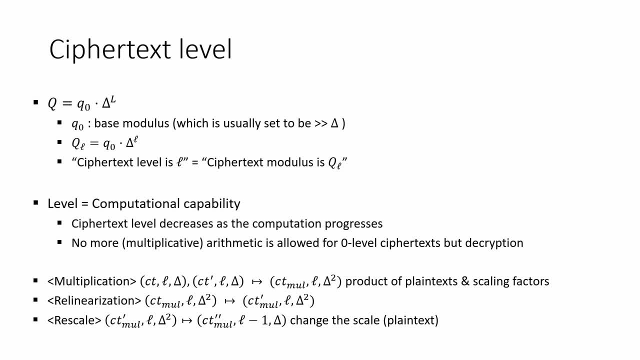 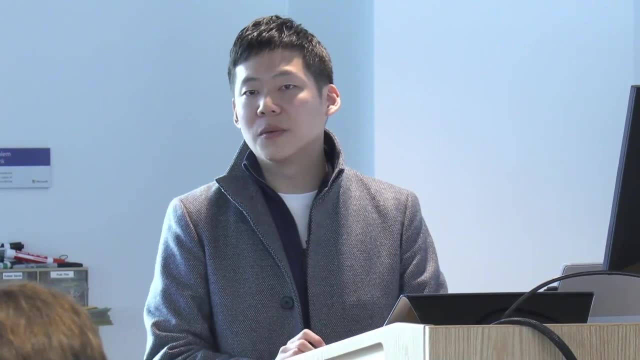 we usually make the use of gradient descent method, But this is really, really expensive in homomorphically encrypted world because we basically repeat a number of iterations for updating model And each of the iteration will consume at least one level. So if you repeat 1,000 iterations, 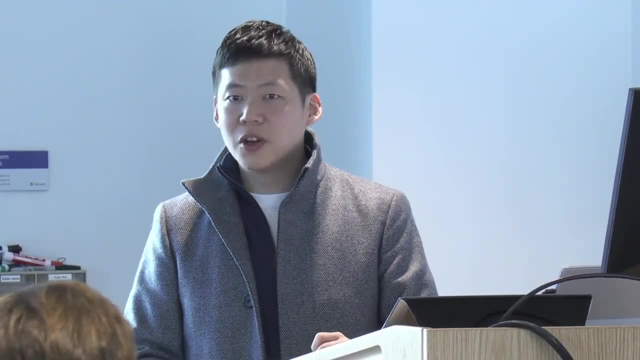 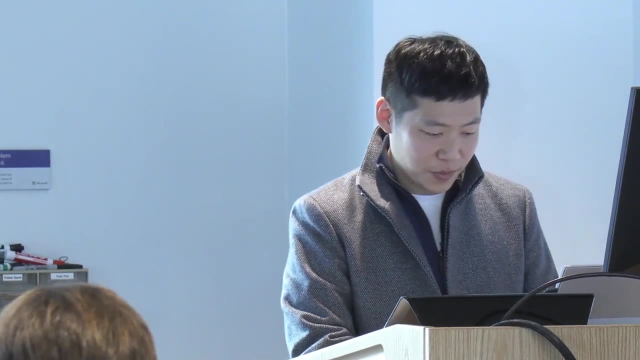 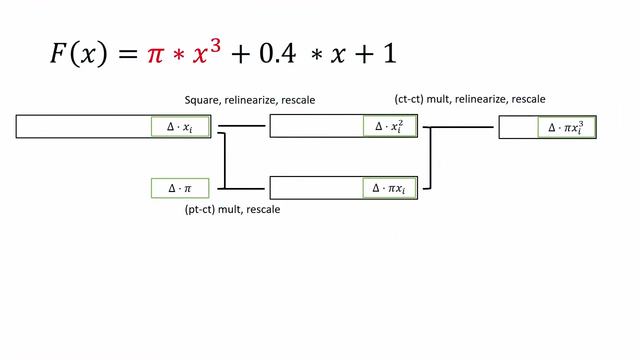 then you should prepare a homomorphic encryption system supporting at least 1,000 level, which is not implementable in practice. OK, So let's get back to this example of source code and focus on the first term: pi times x- cubic. 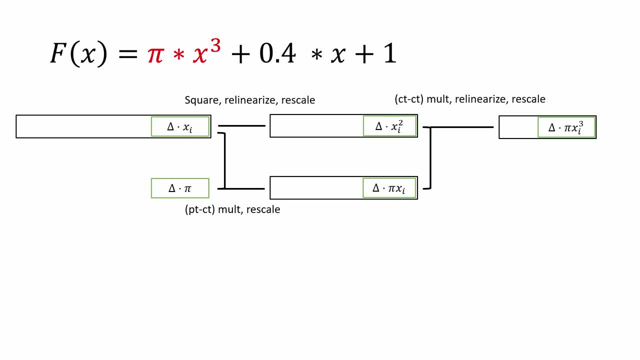 So, since it tests degree four, we can evaluate this term with only depth two system by utilizing these three structure. So we first perform the scaling squaring of the ciphertext, followed by linearize and rescaling operation to obtain this encryption over x squared with scaling factor. 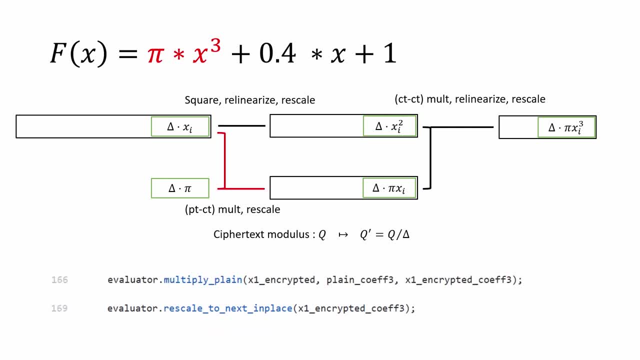 delta. And then we can use plain cipher multiplication algorithm, followed by rescaling operation, to generate another encryption of pi times x with scaling factor also delta, And finally we can multiply them to get an encryption of the first term. These are the term. 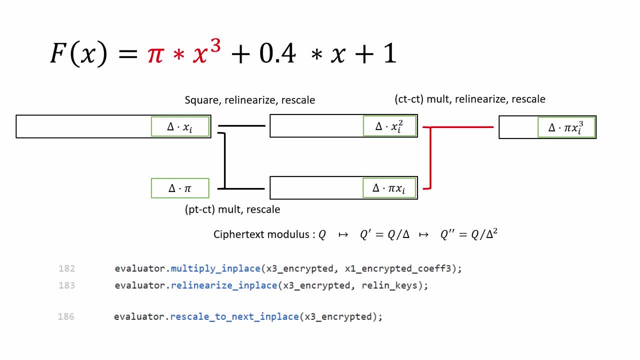 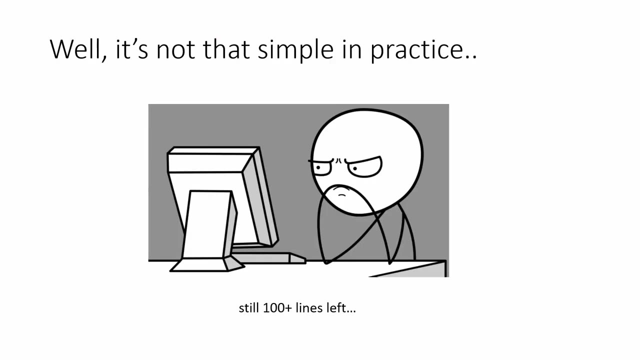 So this is the source code, And we consume the two level And the most difficult part of computation is finish it. So we should be almost done, But actually the source code still have more than almost 150 lines left. So, in fact, what I have explained so far, 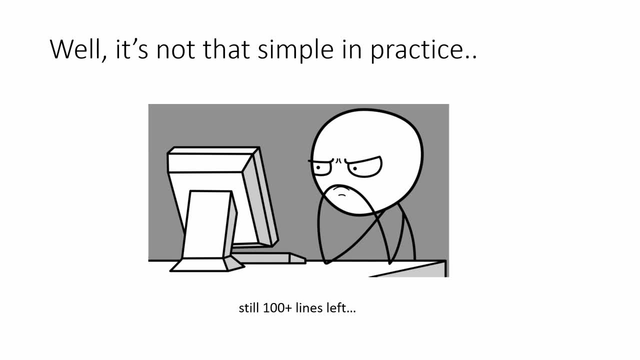 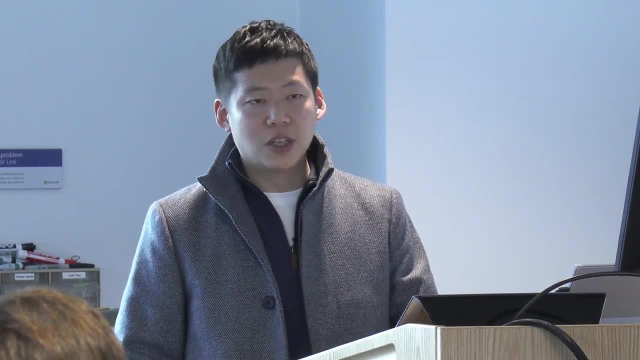 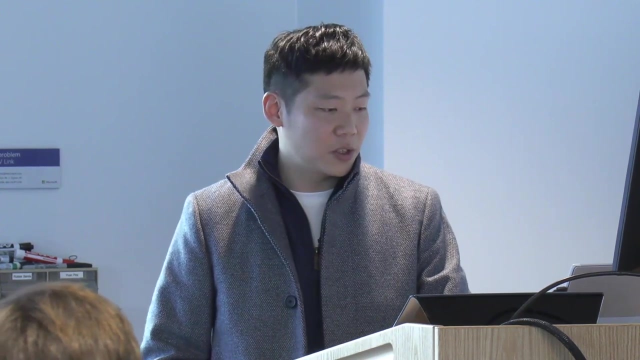 is slightly different from the Algorithms implemented- exactly implemented in our algorithm- because there has been a bunch of modifications and improvements on CKKS algorithm for improving each functionality and efficiency, And some of them are mathematically beautiful or conceptually simple, But we anyway applied some of those optimization techniques. 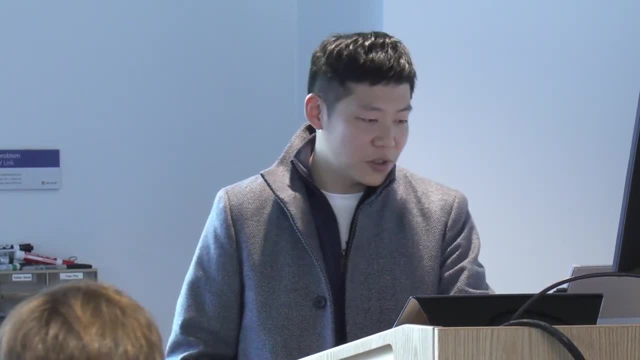 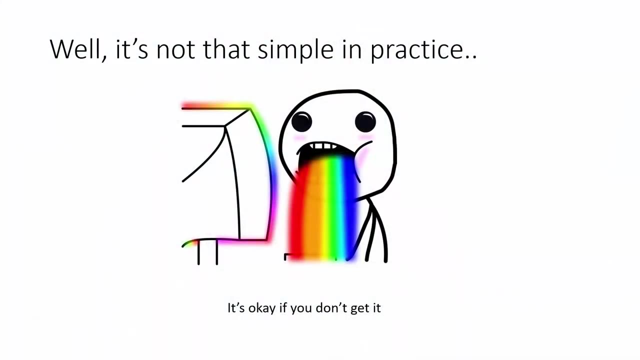 to our library for engineering optimizations. So I briefly explained some some major issues in implementation of CKCAS. but it's fine if you don't understand all the details, because you can still enjoy the power of the CKCAS library without knowing all the details. 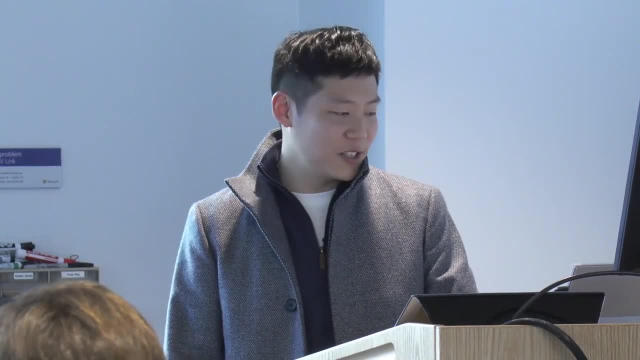 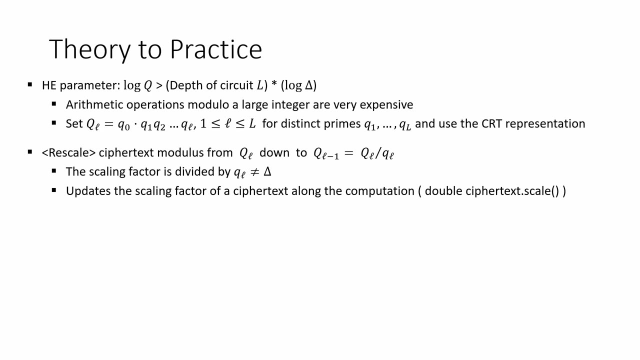 So just understanding is high-level idea is enough. So when you set the parameter for the CKCAS system as I explained, low queue bit size of the cybertext modulus should be larger than the product of depth of circuit L and the bit precision of correctness log data. 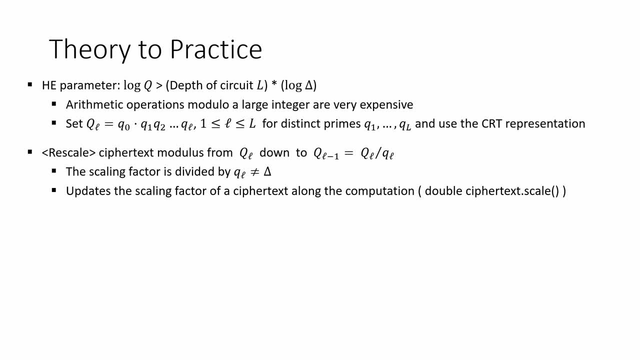 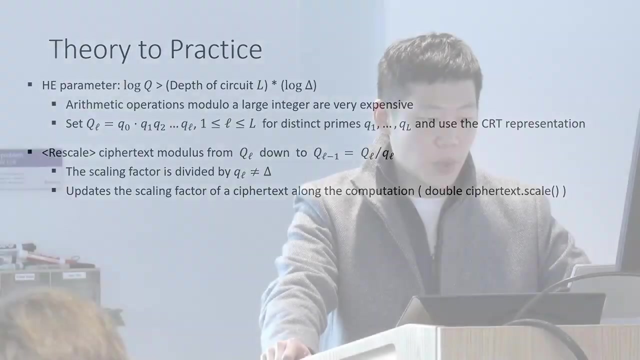 So it could be several hundred or even larger than 1,000 bit in practice. So obviously it is very challenging to implement this high-precision arithmetic on standard computer system which, because we usually work on 64-bit processor but this encryption library require 100-bit arithmetic, modular arithmetic. 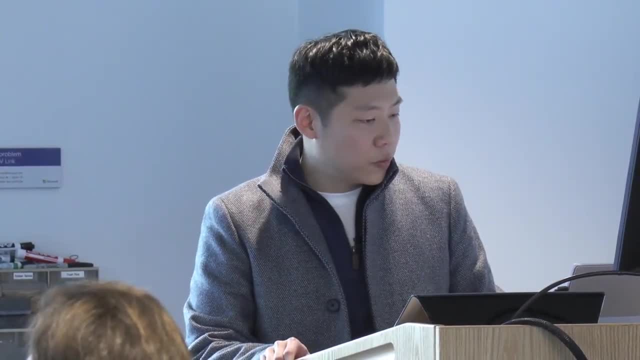 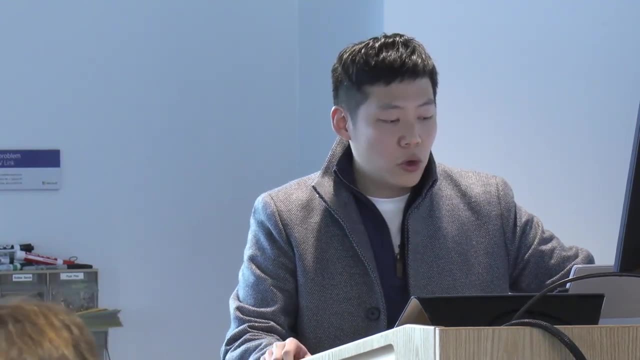 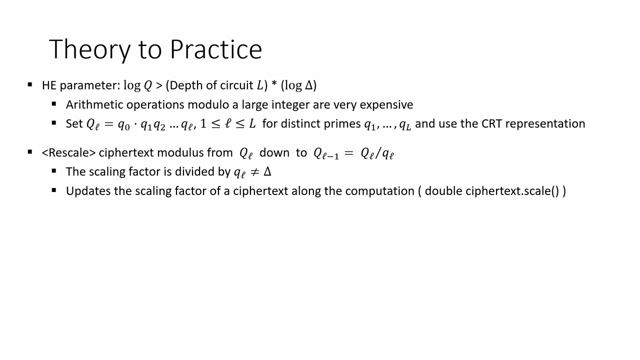 So one well-known solution for this issue is to use the Chinese remainder theorem and represent a single modular Q integer as a two-probe integers in a smaller moduli. So what we call that capital Q was a product of Q0 and delta to the L. 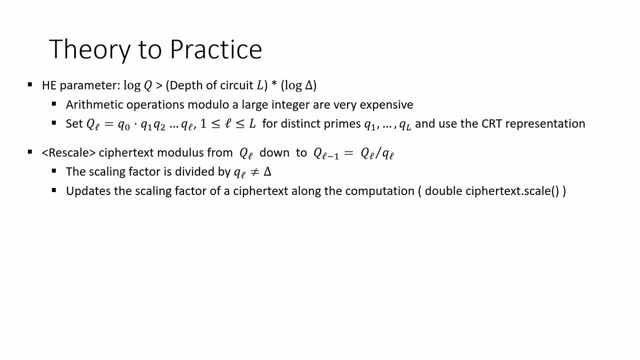 which is not compatible with CRT system. So in our library we search for L distinct primes, Q1 to the QL, and set the cybertext modulus as a product of QIs to support this CRT system. So for arithmetic modular, large QL. 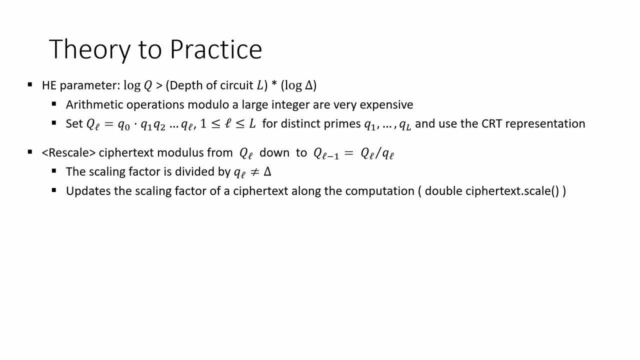 we just store a two-probe small numbers. Each of them can be stored in 64-bit unit, 64 variable, And we can do individual small word-size operations to represent large precision arithmetic. But the thing is, if we play with the chain of cybertext moduli, 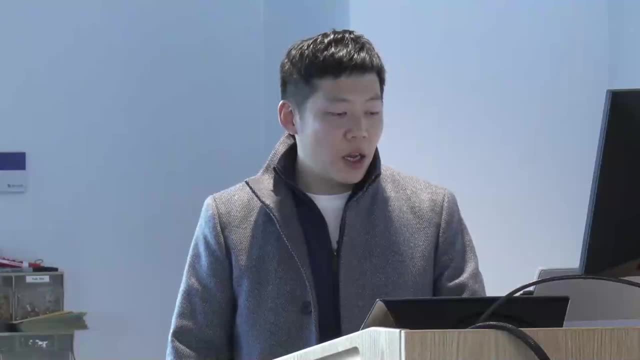 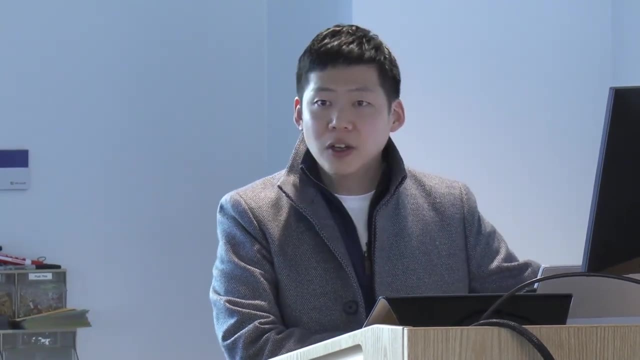 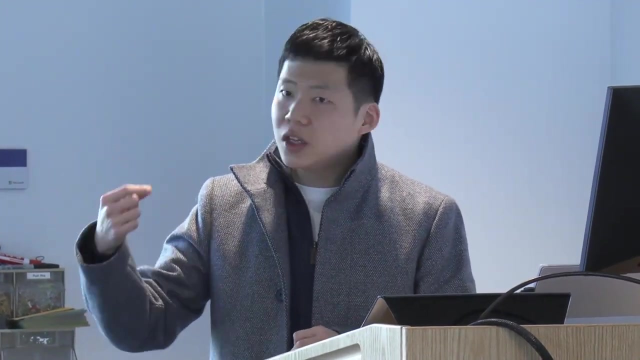 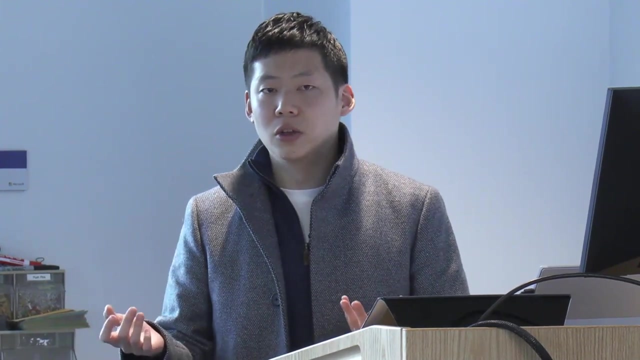 then the rescaling operation at level L basically divides the cybertext and thereby plaintext, by small QL, not by delta. So we can go to only some predetermined cybertext modulus. So rescaling divide. we can't divide cybertext by just an arbitrary number. 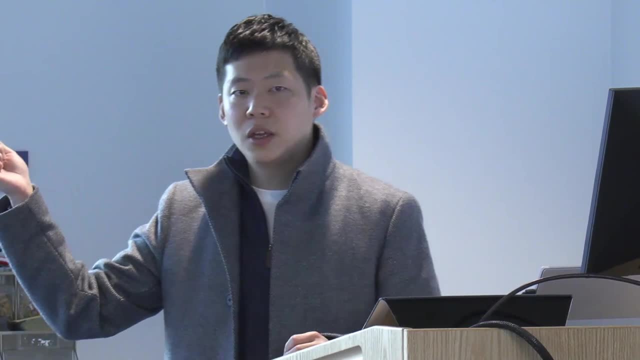 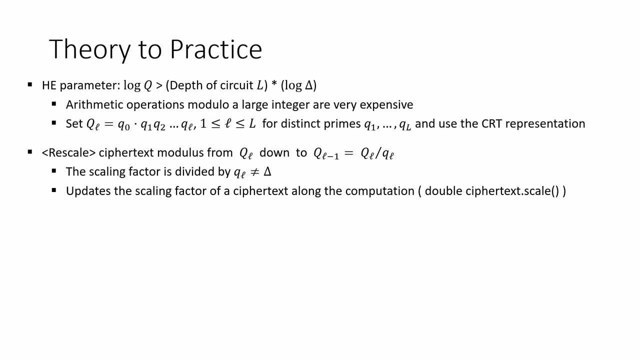 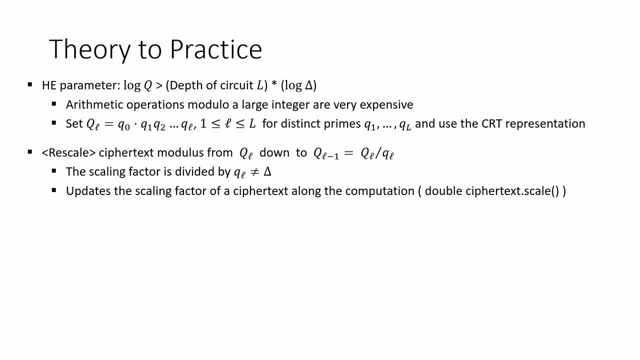 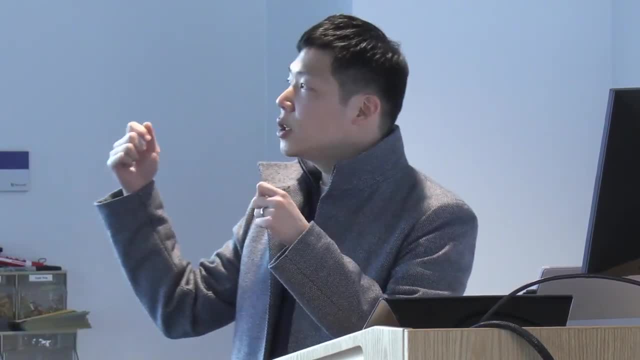 we started off with. we started off with. we started off with. We started from two ciphertexts with scaling vector delta. After multiplication, scaling vector becomes delta squared. But if we rescale this ciphertext by QL, then scaling vector becomes delta squared. 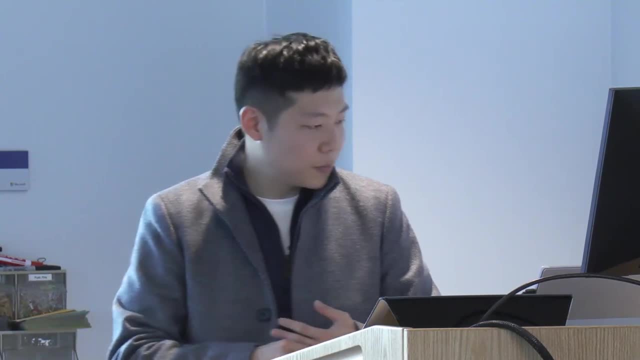 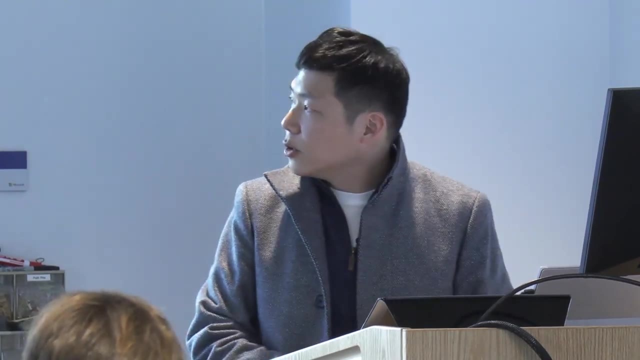 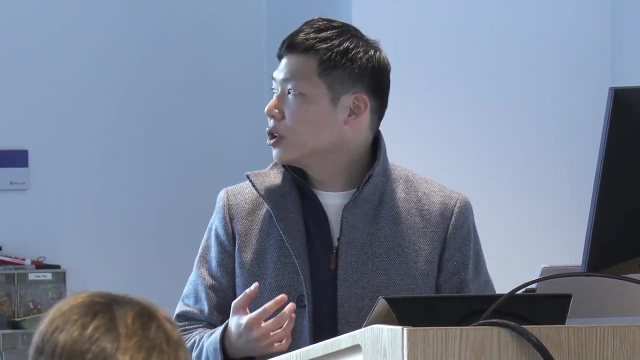 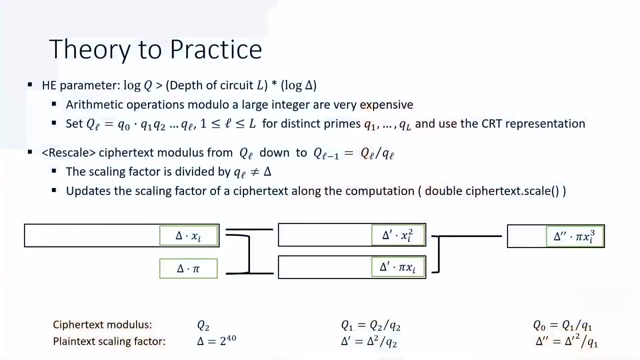 divided by QL, which is different from delta. So there's a ciphertext, that scale function in our library which updates the. So this variable is automatically updated during the computation. We basically keep track of this scaling vector along the computation In the case of this example. first the input ciphertext. 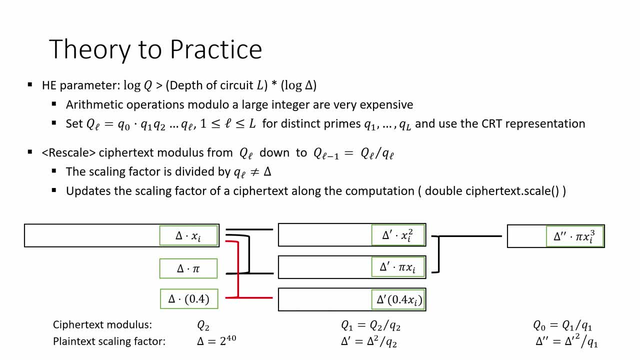 had a scaling vector 2 to the 40.. And after one multiplication its scaling vector becomes Delta prime, which is delta squared divided by Q2.. And after one more multiplication its scaling vector would be delta prime squared divided by Q1.. 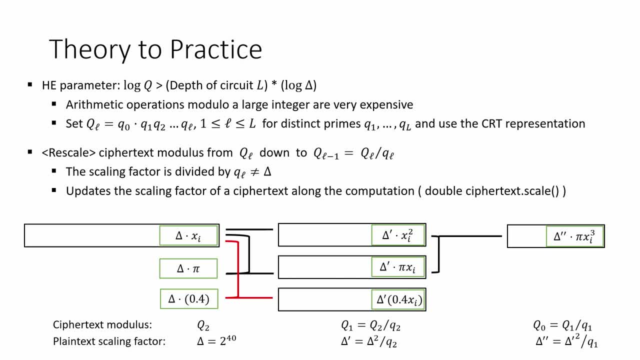 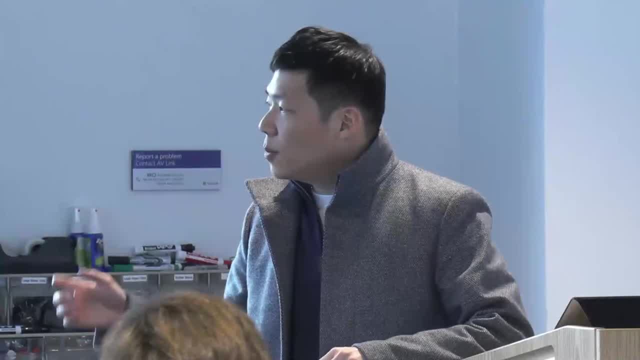 It's again different from delta prime. But the problem is the second term was 0.4 times x, which requires only one depth to evaluate. So if we prepare the encryption of second term, 0.4 times x, then we obtain an encryption of 0.4.. 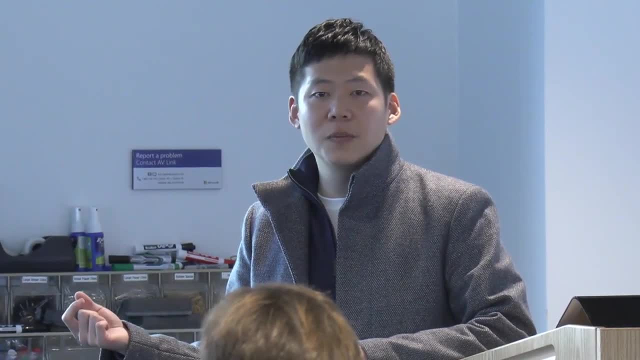 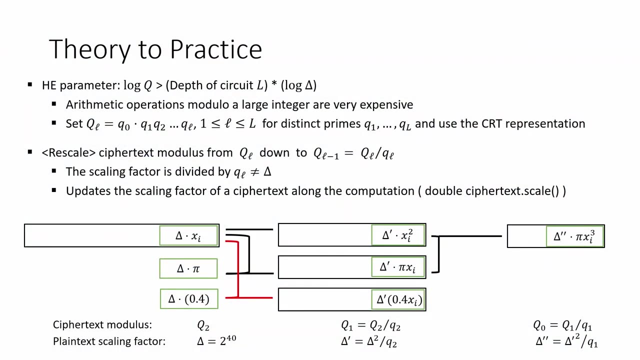 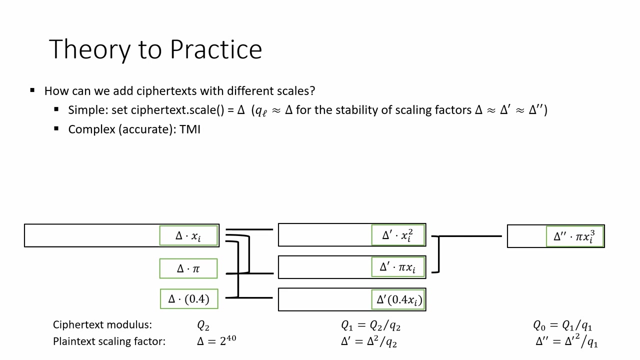 0.4 times x, 0.4 times x for x, with scaling vector delta prime, And we showed that two ciphertexts with different scales- delta prime and delta two prime- And this is not trivial. So a simple solution of solving this issue. 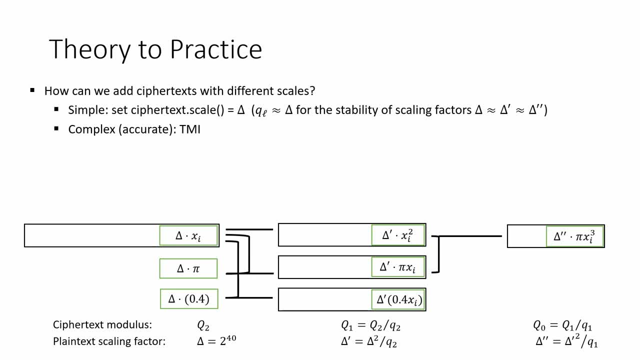 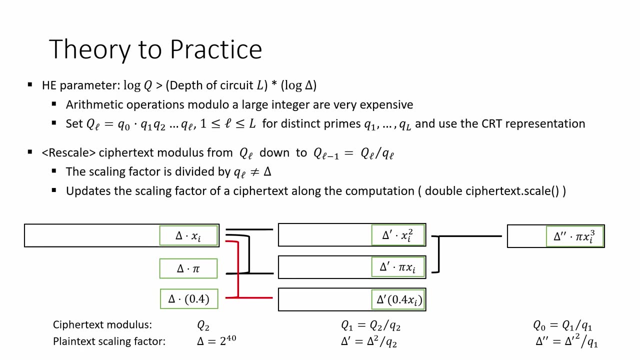 is just set scale of all ciphertexts as delta, bimanually. It is fine because in the parameter setting- excuse me, in the parameter setting, when we search for these intermediate primes from q1 to qL, we try to make them as close. 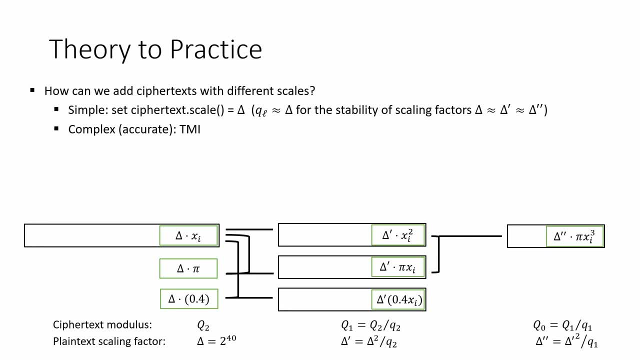 as to the scaling vector delta. So division by qL is approximately equal to division by delta. So it's fine To set the scaling vector as delta. delta prime and delta two prime are slightly different from delta, but they are almost close to each other. 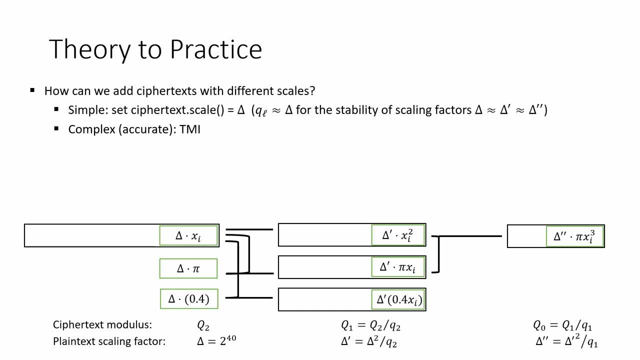 So you will lose some precision, but it's generally fine. And there is another method which, without precision loss, you can just consume one level to change the scale of a ciphertext. but I'm not going to go into details, It's too much. 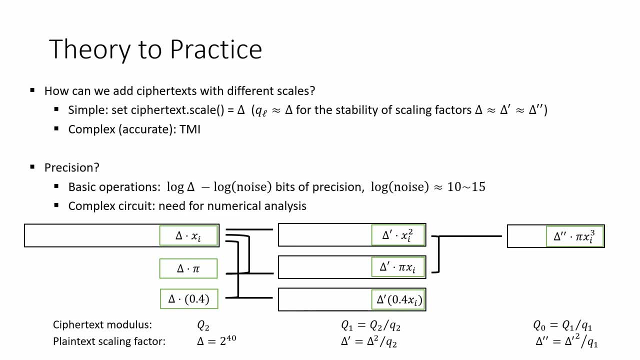 And the precision is another issue when you we should think about. So basic operations such as homomorphic multiplication or rotation introduce some small noise. So we could say the bit precision of basic operations are log, delta, minus log noise And the bit size of noise is usually between 10 to 15. 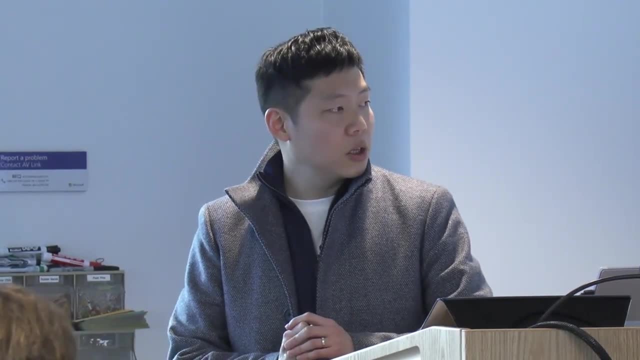 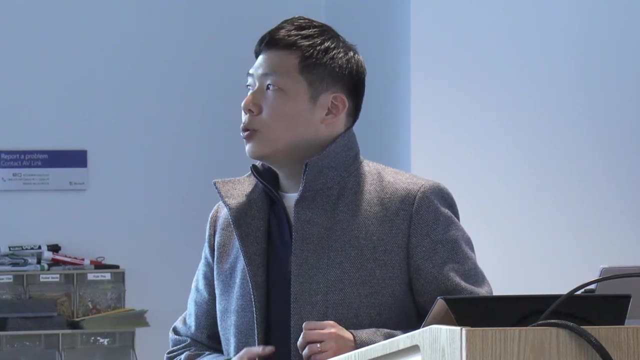 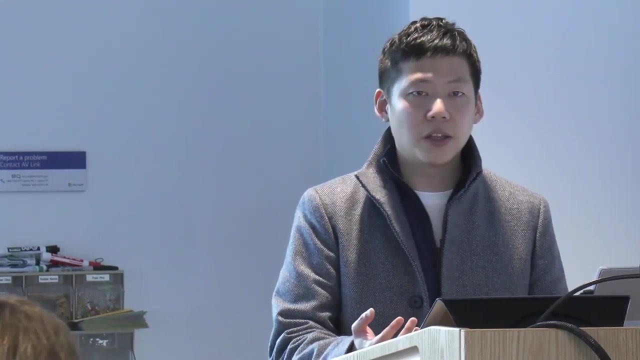 in practical parameter setting. So in our example log delta was 40. So we could say you preserve roughly 25 to 30 bits of precision after Reddick's point when you encrypt plaintext or perform some arithmetic. Of course, in general case when you evaluate, 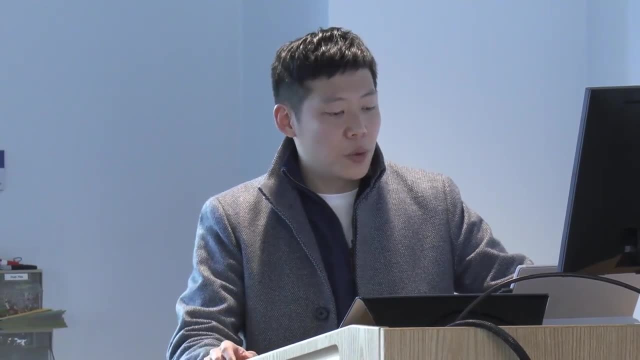 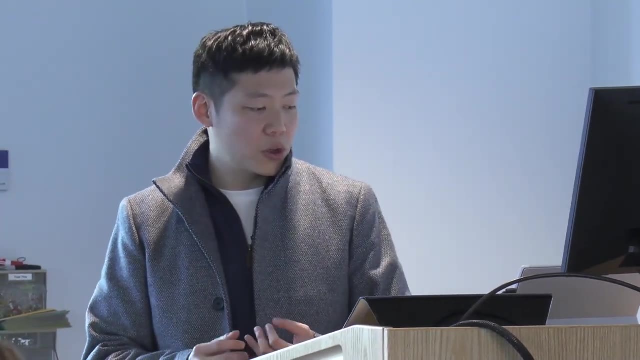 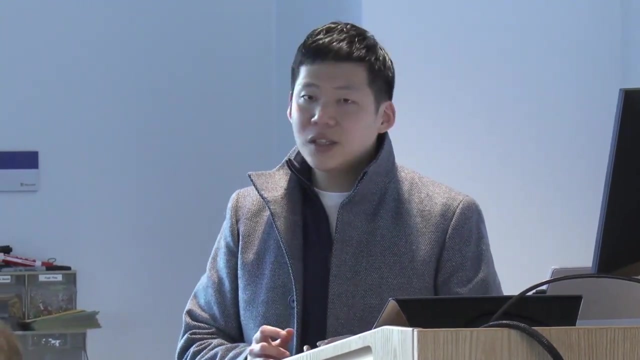 a complex circuit by representing it as a composition of basic operations. it's generally very difficult to estimate the accuracy of the result. You probably need a new microanalysis to make a good estimation for precision. But it's not just an issue of encrypted computation. 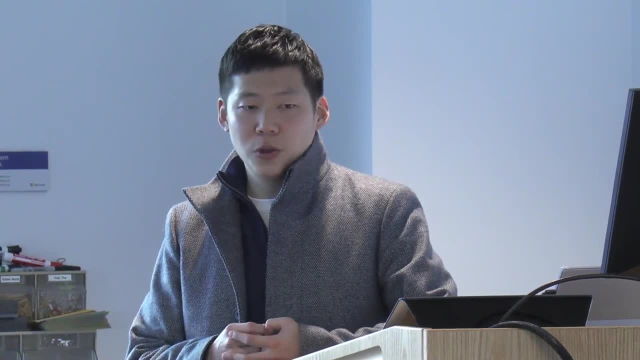 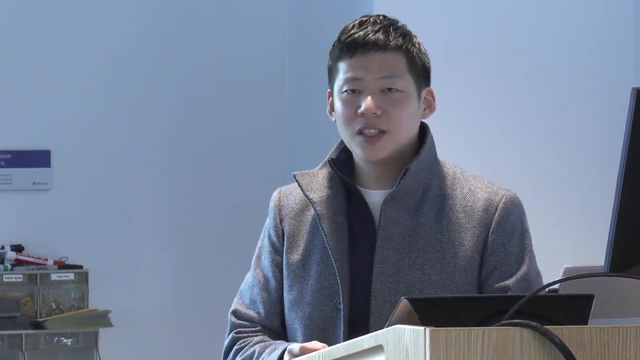 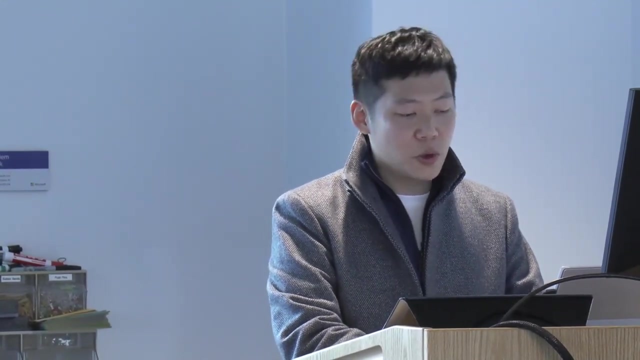 Even in just plain computation, where you use a double precision for calculating some approximate circuit, it's not easy to estimate the precision of the result. So we have almost the same issue here. But of course you can. Of course you can always increase data. 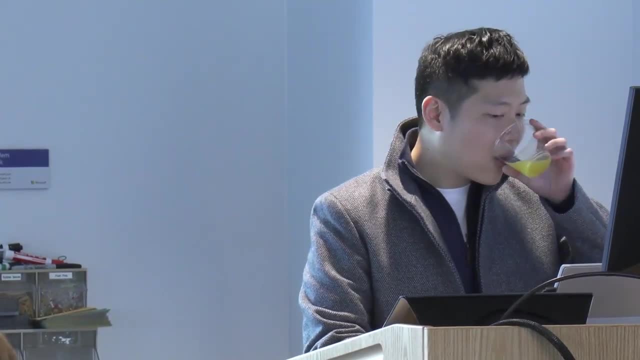 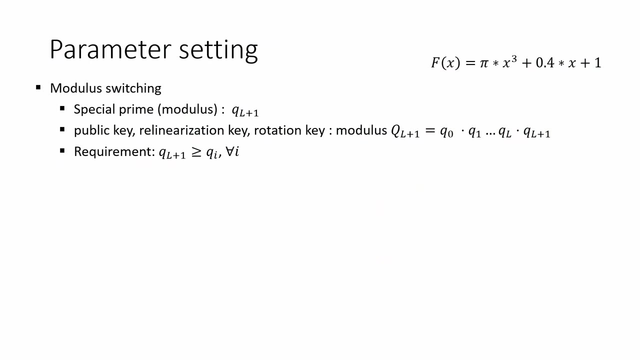 to achieve better precision, And modular switching operation is basically used during linearization or encryption. So there's a special prime, There's an integer called the special prime, which is denoted by q? l plus 1.. q? l plus 1.. 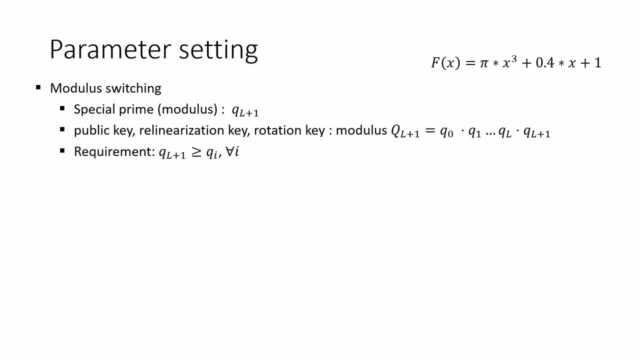 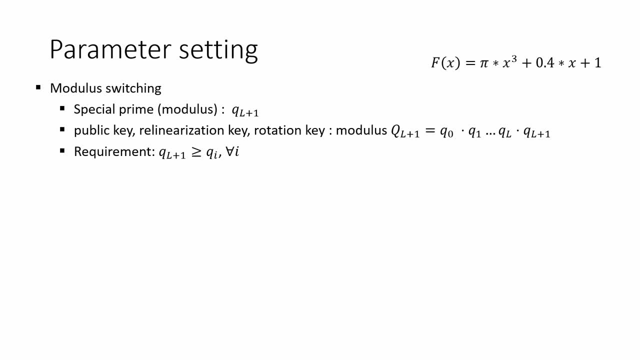 than all other primes. q, i Too many is the noise growth of operation, So I'm going to skip some details, but just remember that there's just a special prime which and it is not for ciphertext, And in this example code I'm going to skip some details. 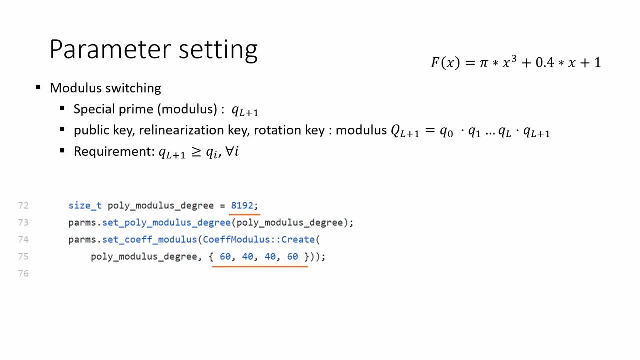 And the ring dimension n is 2 to the 13.. And for the security region, log q l plus 1 should be bounded by 218 to ensure the security. And since we are evaluating the circuit of depth 2, we basically need four primes. 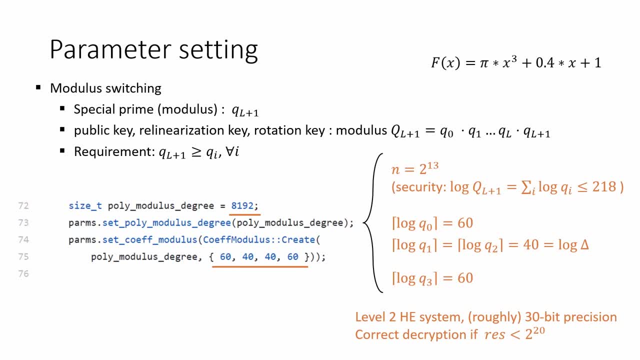 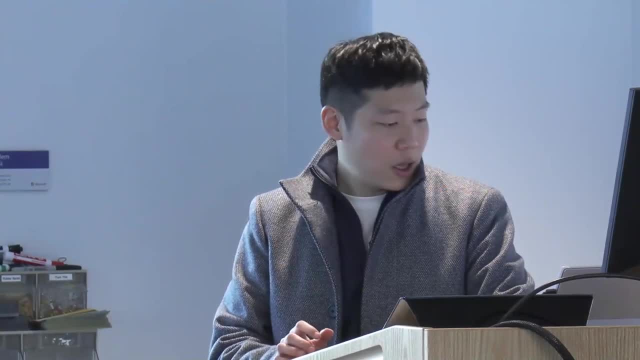 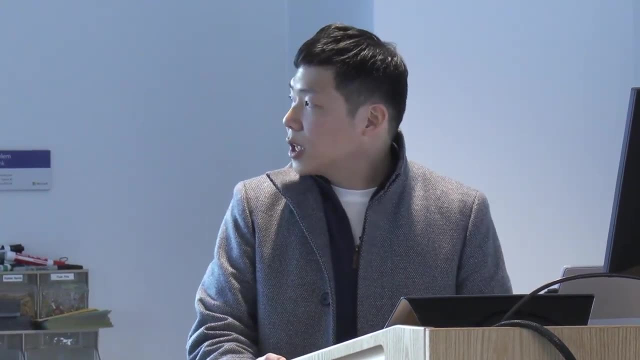 Because q j 1, base prime, q 0, and two intermediate primes, q 1 and q 2, for rescaling. q 1 and q 2 for rescaling And the special prime q 3 for modular switching technique. Here the size of q 1 and q 2 are 40,. 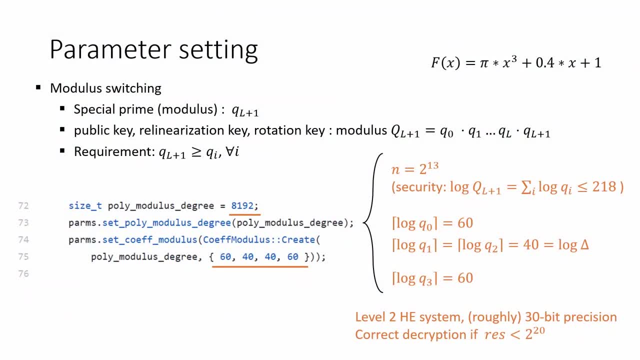 so that they are approximately equal to the scaling vector delta 2 to the 40. And q 0 is 60. And q 0 is a 60-bit prime, so that we can decrypt the ciphertext correctly as long as the computation result is smaller than 2. 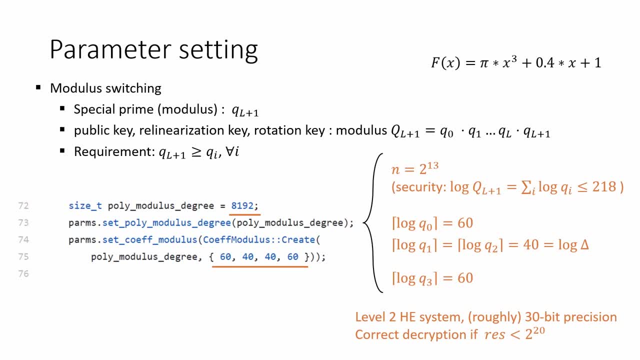 to the 20.. So message is already. It's scaled by 2 to the 40. And plaintext should be bounded by 2 to the 60, meaning the actual size of message should be bounded by 2 to the 20.. 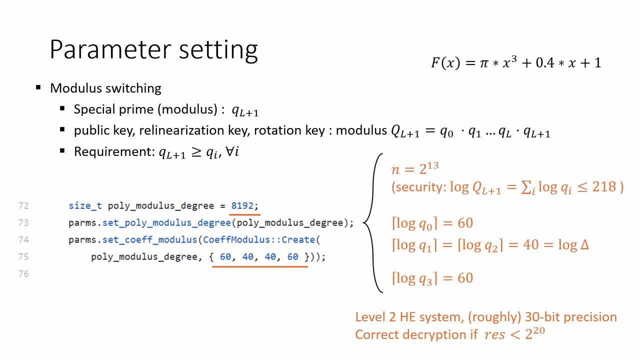 But we are just evaluating this simple polynomial on small real numbers which will definitely be bounded by 2 to the 20.. And finally, the special prime q 3 should have maximum size also 60 bits, And we can double check that, the bit size of the largest modulus. 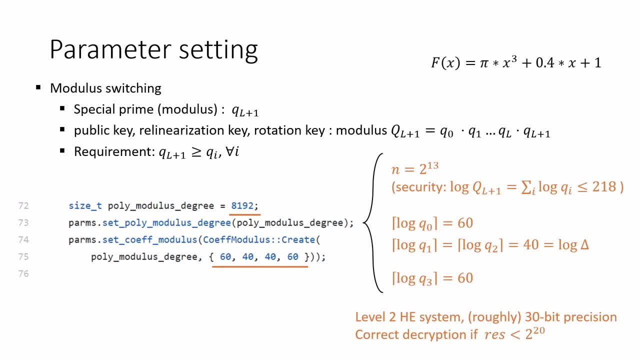 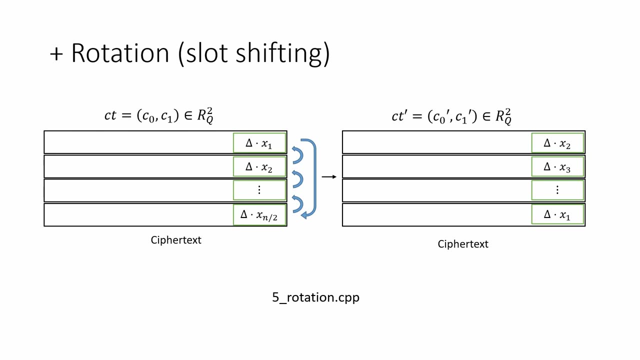 the sum of bit size of all small qi's is 200, which is smaller than 218. So this system is secure. I didn't explain this rotation because rotation is not necessary for polynomial evaluation, but this operation will be used in some later sessions. 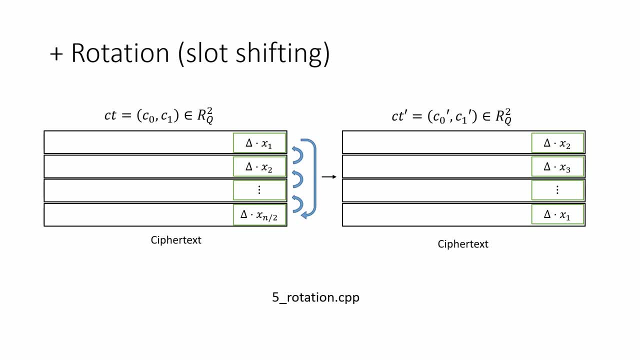 So suppose that you want to compute something using plaintext values located in the different slots. In this case you can utilize this rotation function to publicly rotate the encrypted plaintext and obtain shifted plaintext and compute some functions on the values in different plaintext slots, And you can check out this. another example code: 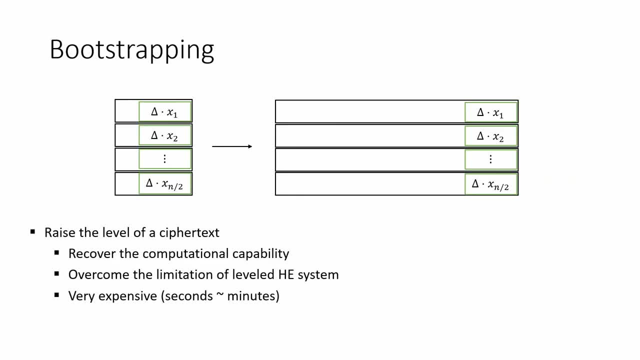 And this is the last slide, And as I mentioned earlier, a ciphertext has a final level, L, and no more computation is allowed when its level becomes 0. So bootstrapping is a public algorithm which generates a high-level ciphertext encrypting the same plaintext. 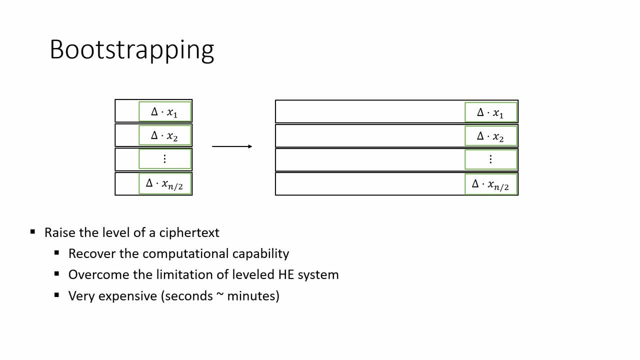 And you can do further computation on this refreshed ciphertext. So it's basically public conversion from level 0 ciphertext to higher level ciphertext. So we can combine this bootstrapping with a leveled CKCAS system to obtain a fully homomorphic encryption which supports the evaluation of an arbitrary. 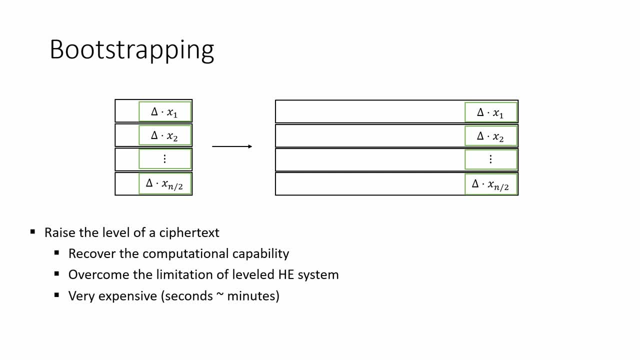 circuit without limitation of its steps. You can just repeat evaluation and bootstrapping as many as you want. Unfortunately, this CKCAS bootstrapping is not yet available in SEO, but we are working on it, So it will be definitely Released in a later version in the future, hopefully. 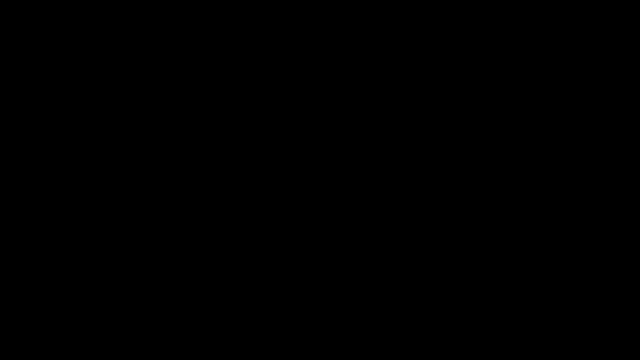 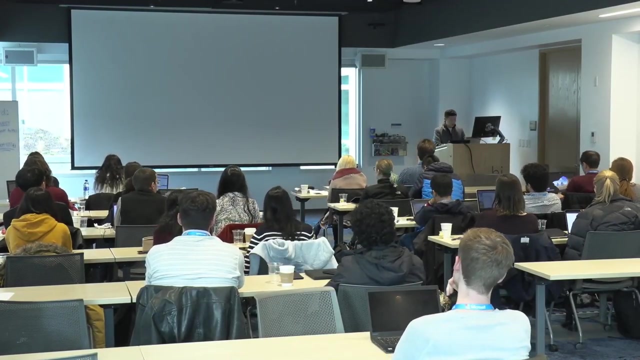 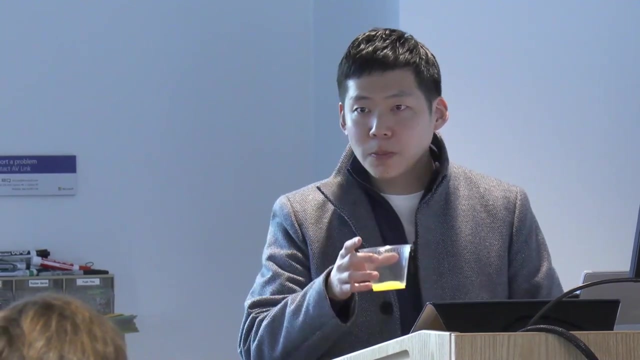 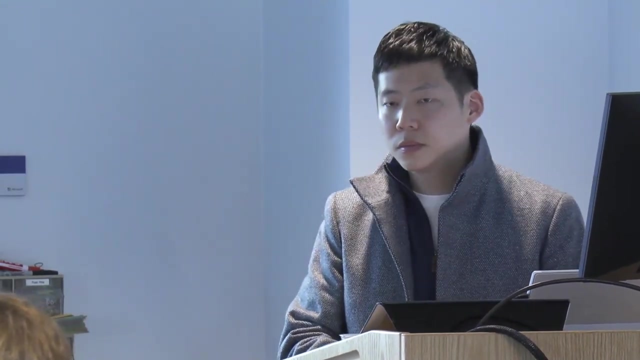 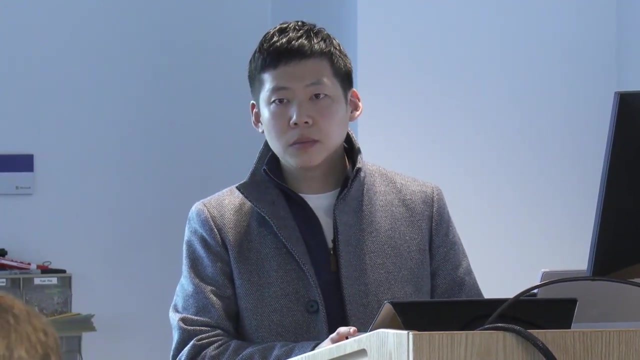 Yeah, Okay, Thank you for listening. Are there any questions? So for the scaling factor, the like BGV rescaling just like switches, the modulus that is in the scaling factor. I guess this, by restricting the limbs, to like be close to this power of two. 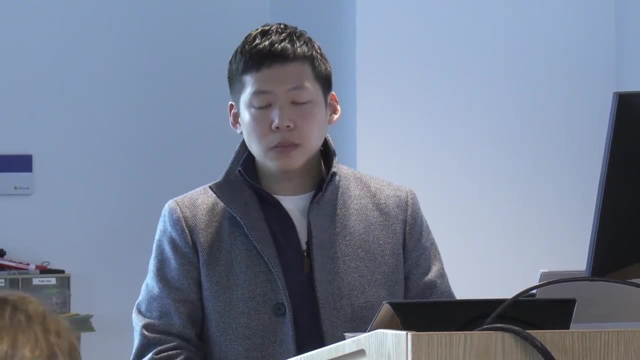 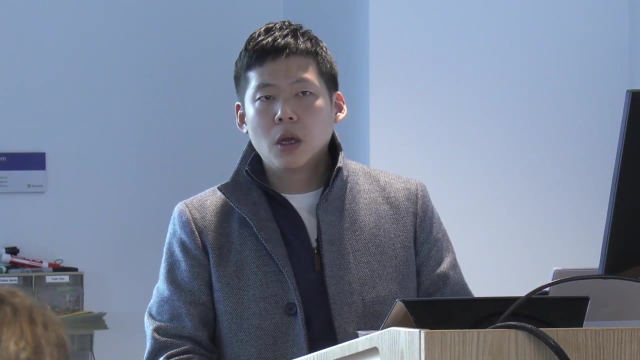 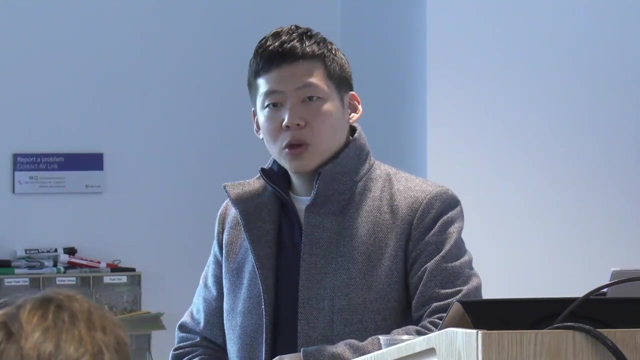 it kind of like limits your selection or like your error grows as the number of limbs grows. Is there a way to like get the BGV rescaling technique to work with this? So technically this rescaling algorithm is almost same as the modular switching technique of BGV. 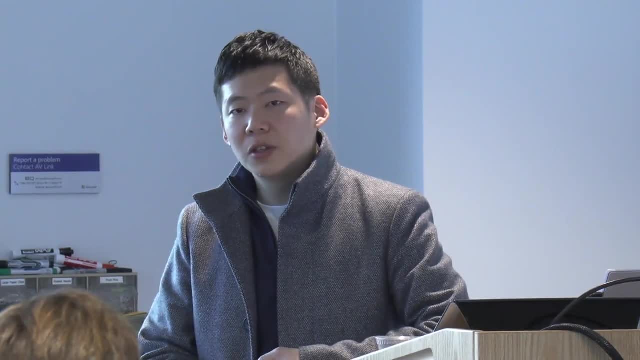 Okay, So technically, this rescaling algorithm is almost same as the modular switching technique of BGV. So, technically, this rescaling algorithm is almost same as the modular switching technique of BGV or BFV scheme, but the purpose is different. So in the case of BGV, 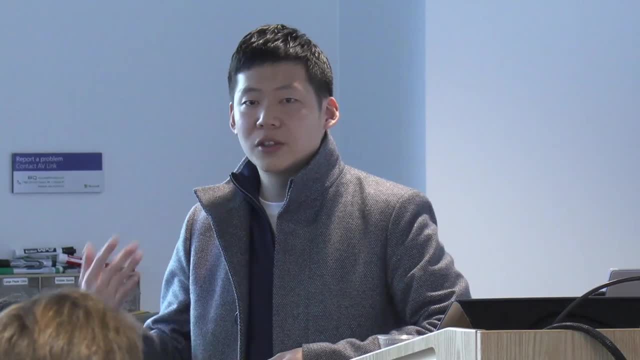 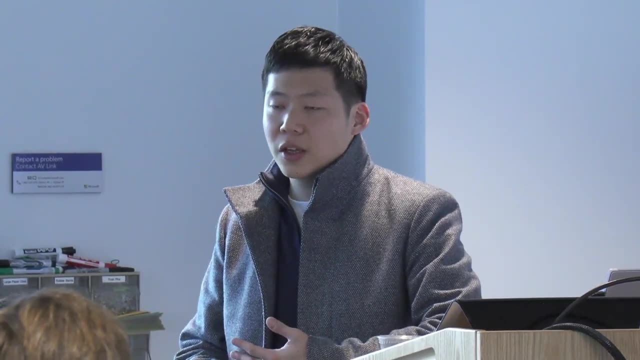 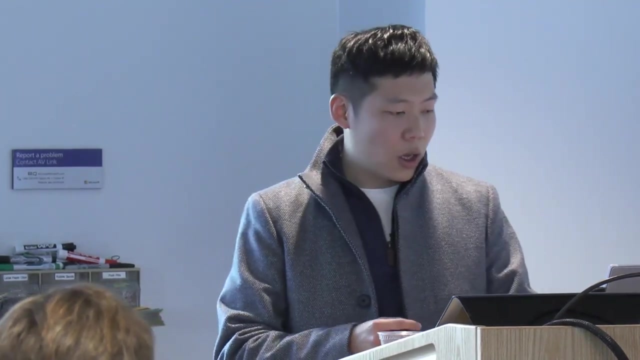 you basically use modular switching operation to reduce the size of noise, but you just preserve the plaintext Up here. this rescaling changes the representation of plaintext, So as in floating point representation, So cyphertext before rescaling and after rescaling. 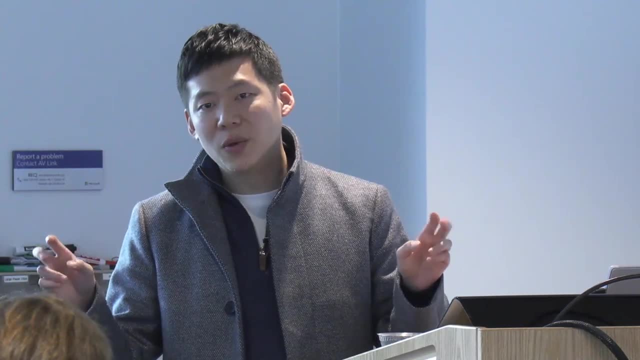 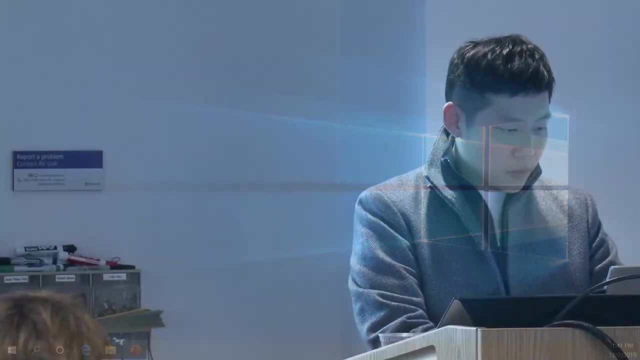 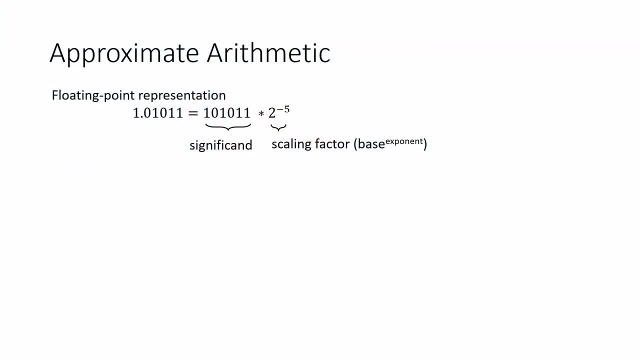 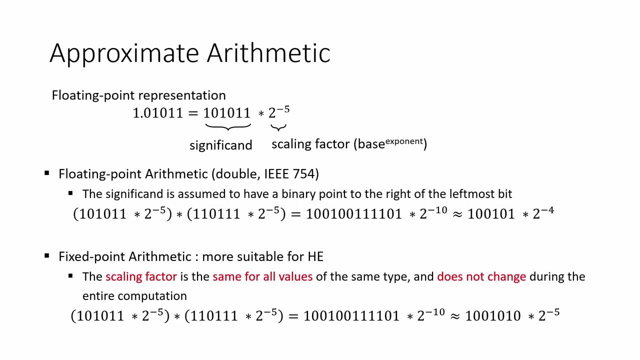 are actually two different encryptions of the same message with different scale. Okay, So like a. okay, So in this last approach, approximate equality. these two numbers are actually two different representation of the same number, So we divide this significant by scaling factor. 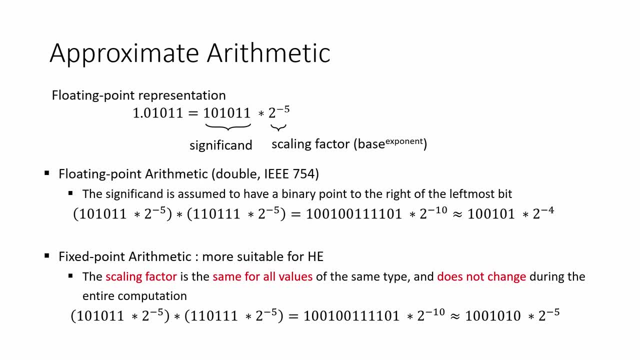 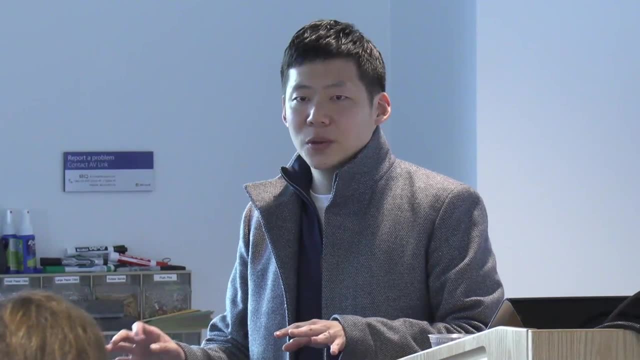 two to five here to make a trade-off between efficiency and precision. So since CK case rescaling has this functionality, the goal of this CK case rescaling is not to manage the noise. we don't care about noise because noise is always a part of plaintext. 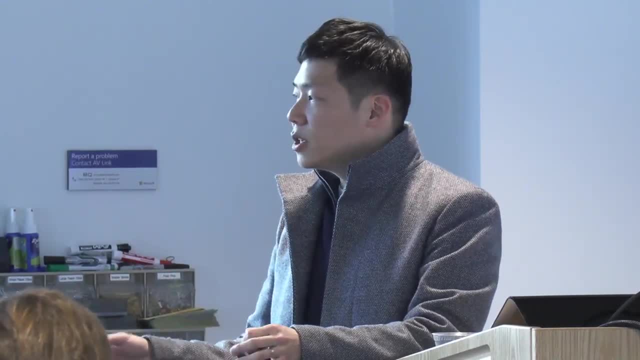 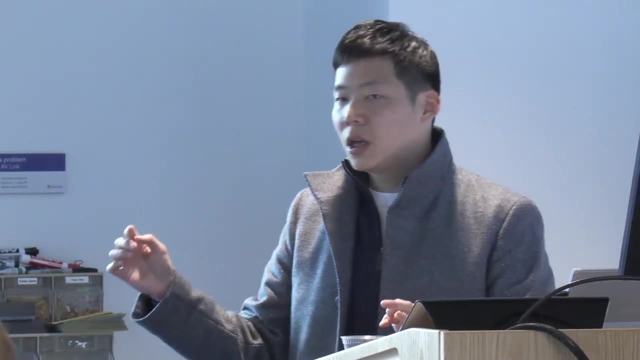 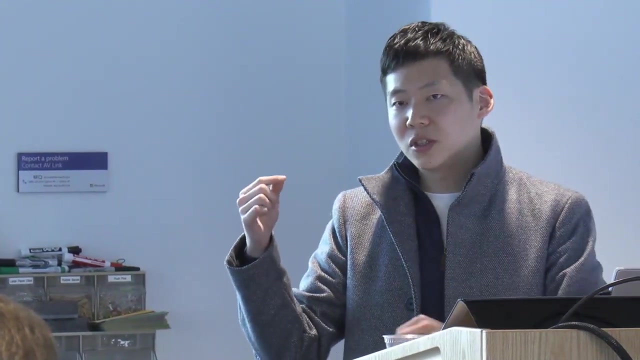 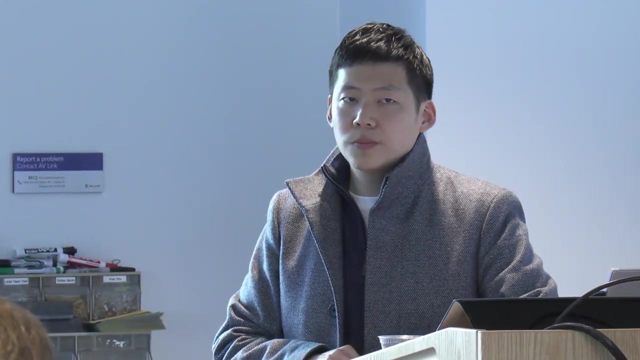 We just consider significant. But the size of significance is increased after some multiplication and we should cut off it. So basically, that's why the cyphertext modular chain depends on its related to the functionality of this rescaling in CK case. So 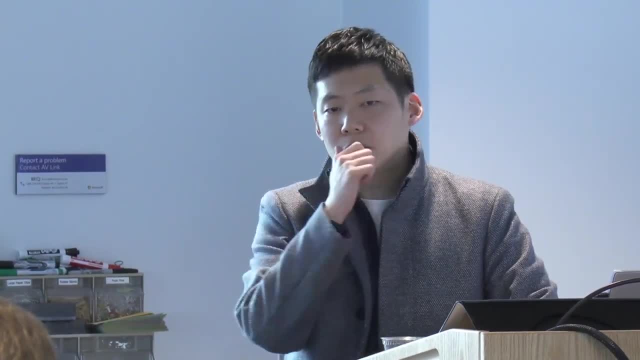 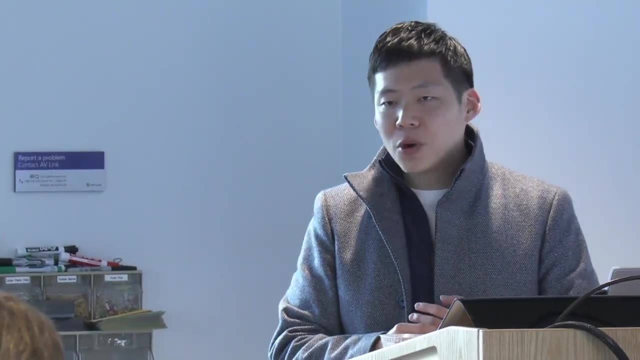 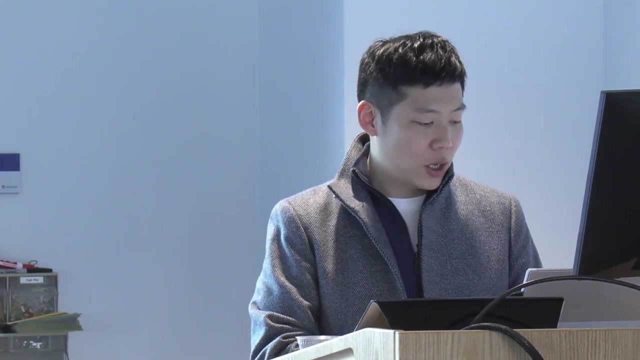 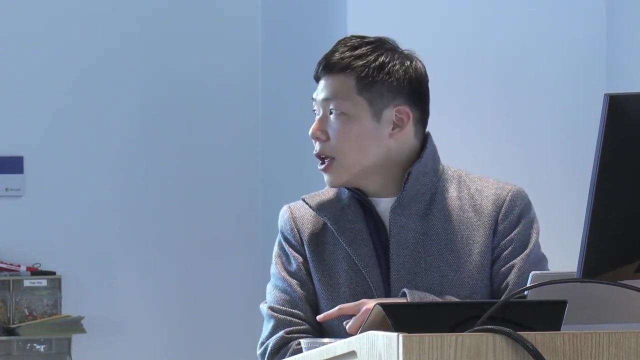 yeah, so I would say we are already using the same technique to answer your question, but the purpose are different. So that's why we have some additional requirement on these primes. So that's why in the original paper we couldn't use this RNN system, because we had to keep this mathematical simplicity. 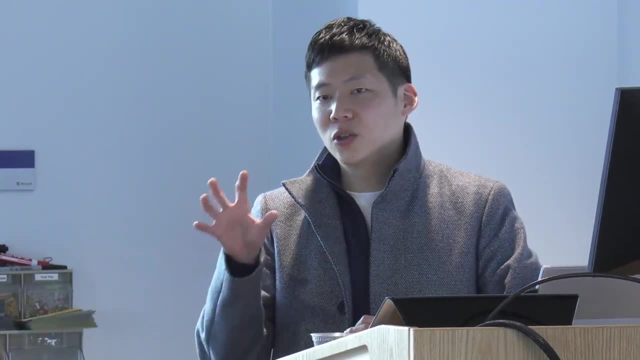 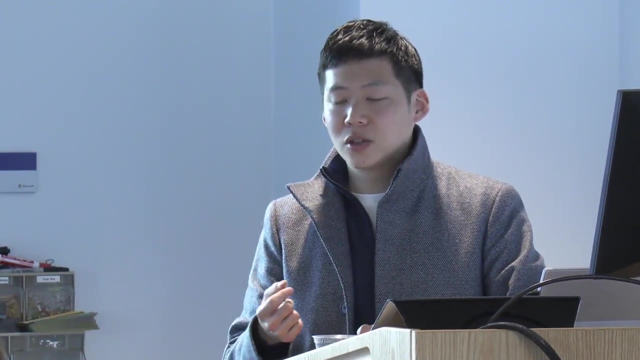 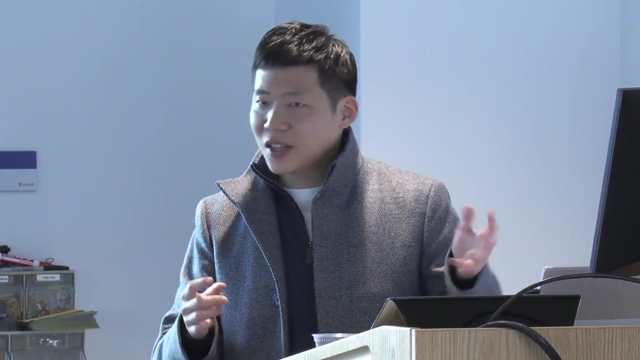 So Q was set to be Q zero times delta two, So the L, to keep the same base. But in later papers we slightly modified this scheme by searching for some primes approximately equal to delta. So to take advantage of both words from engineering: optimization of BGV. 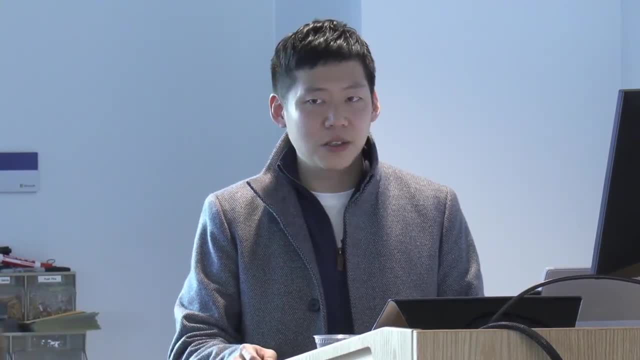 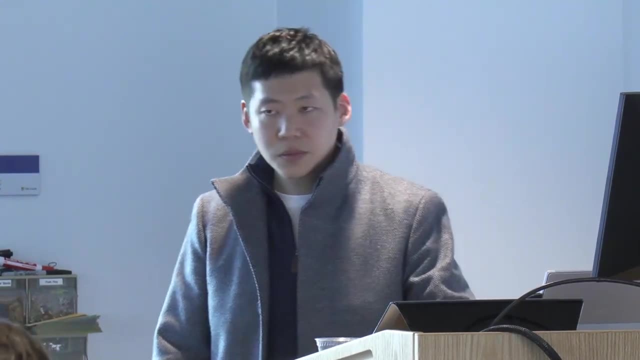 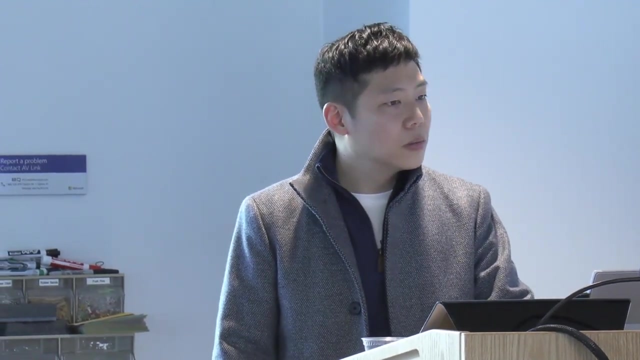 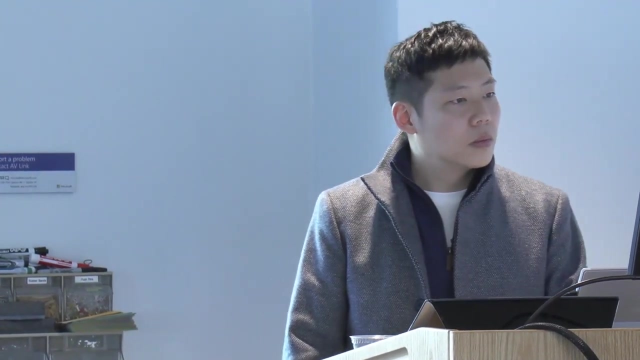 and still keeping the functionality of CK. Yeah, So for the decryption step. So you just take the like B minus AS mod, the cyphertext modulus, and then there's no plain text modulus that you need to reduce by. is that right? Yeah, That's a good question. 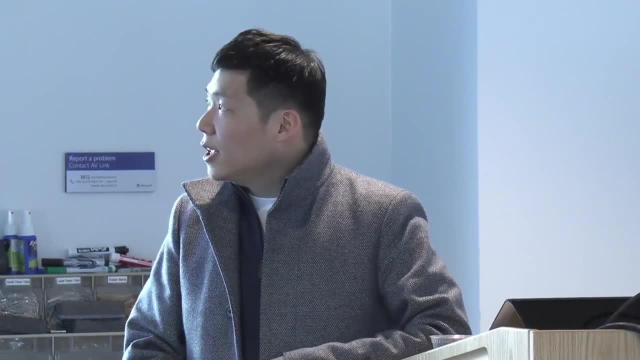 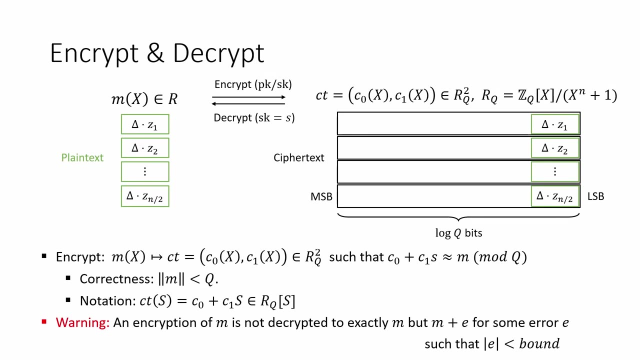 So I didn't clearly explain what is the plain text space of CK case. So roughly, the plain text spaces just are set up. Yeah, So roughly, the plain text spaces just are set up. Yeah, So roughly, the plain text spaces just are set up. 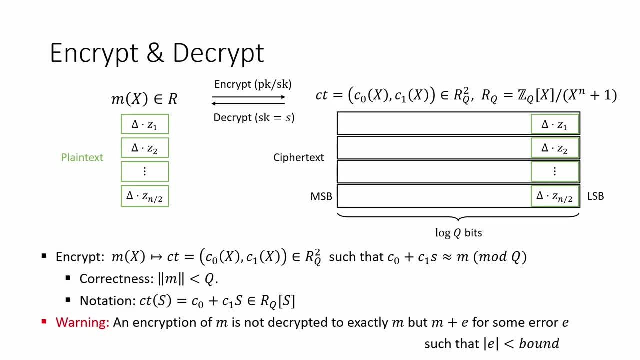 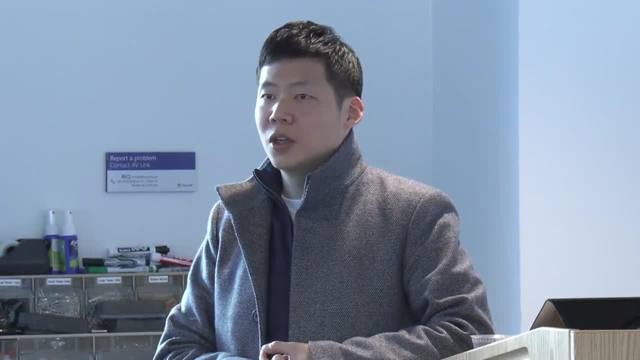 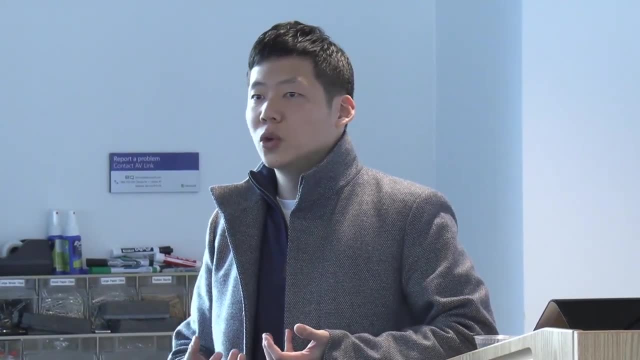 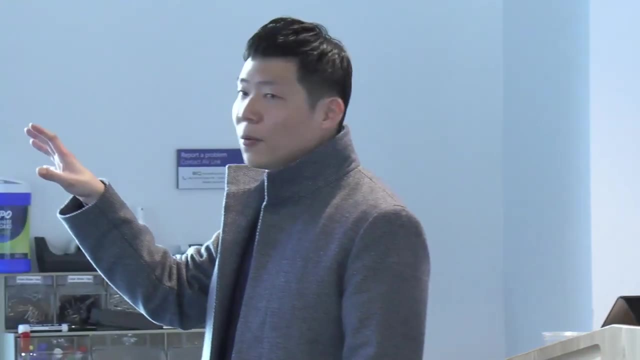 any polynomials. but for corrected decryption the size of plaintext should be bounded by ciphertext modulus. So there's no plaintext modulus in this scheme. So you just work on just a polynomials with no characteristic. Yeah, But of course ciphertext itself has modulus Q. 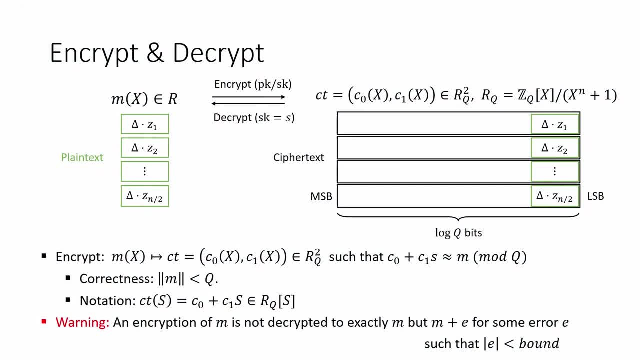 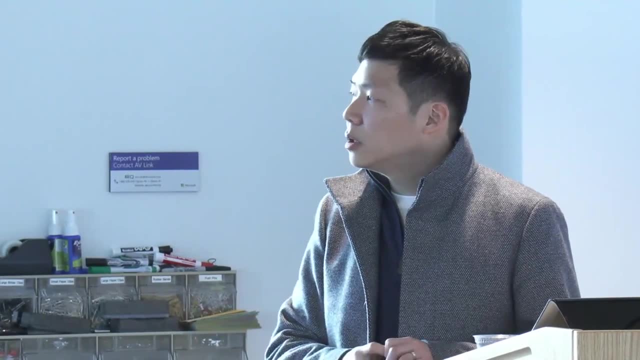 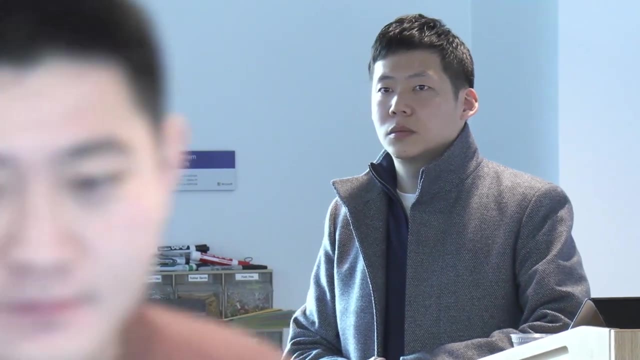 So you can recover plaintext by computing c0 plus c1s and take modulus Q. If you generate the ciphertext correctly, then the result would be much smaller than Q in general. Okay, Thank you. To follow up on the decryption, so the plaintext: 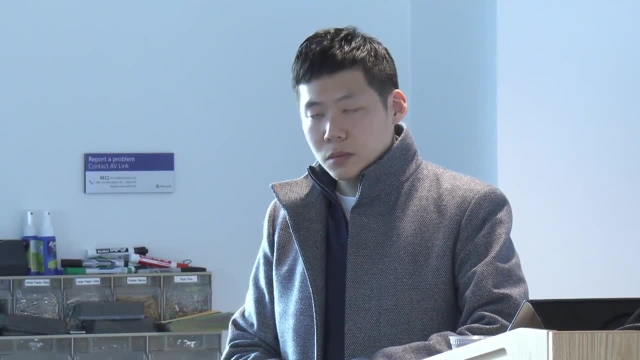 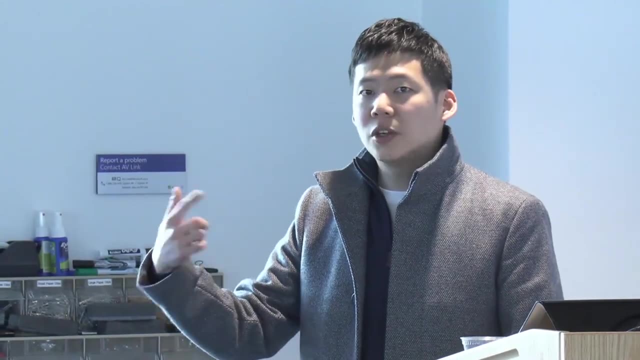 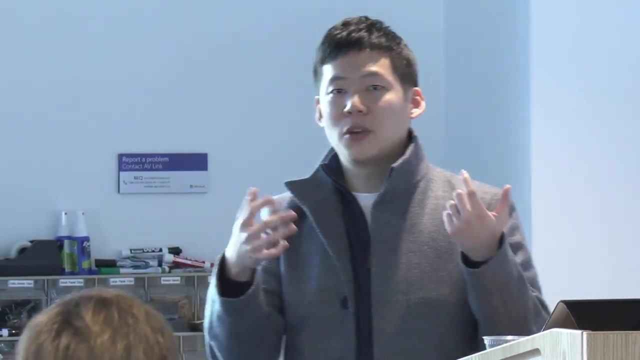 it needs to be smaller than the last Q0, right, Not the full initial big Q. Yeah, So as computation progresses, the ciphertext modulus decreases and we don't know how the size of plaintext will change. It depends on input size and circuit. 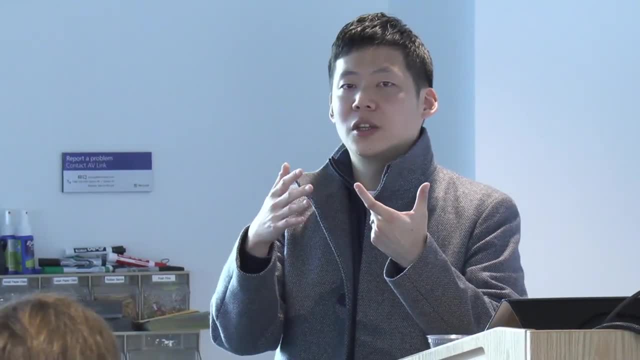 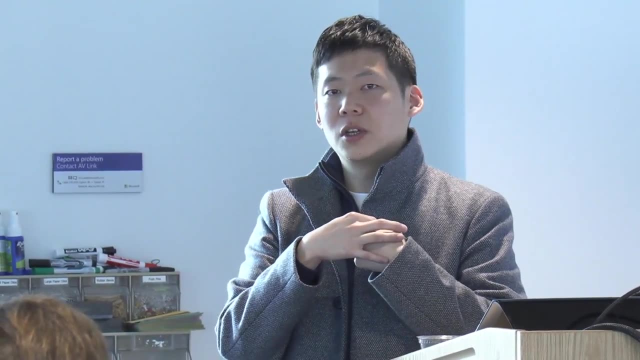 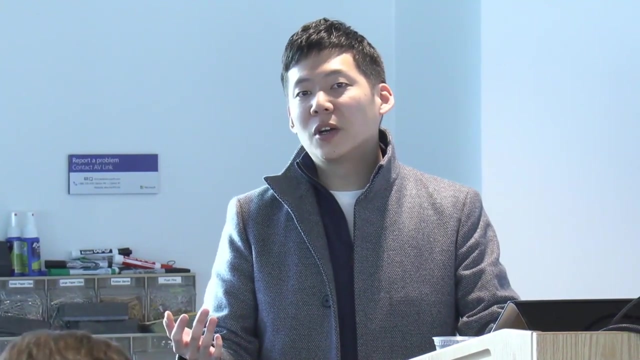 But anyway, the value should be always smaller than ciphertext modulus at lower level to ensure the correctness. Okay, So you're right. So that's why we said Q0 larger than delta, Because, after consuming all levels of our homomorphic encryption system, 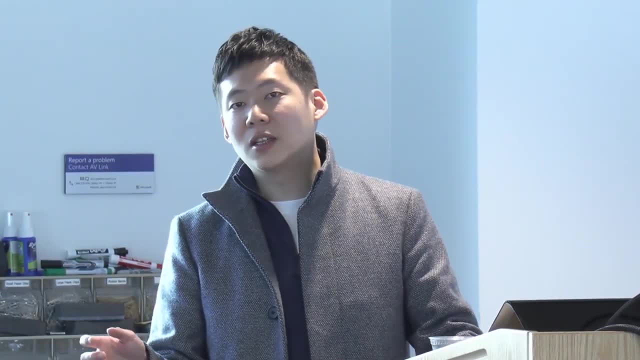 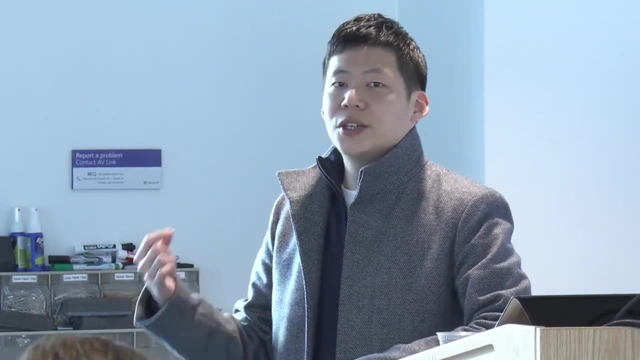 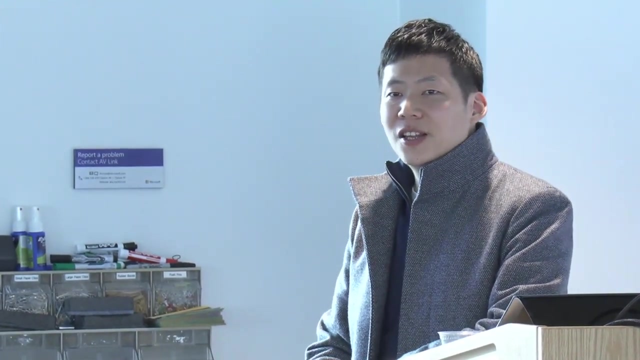 you still have a modulus Q0, which is much larger than delta, So that your message, scaled by delta, would be still smaller than Q0. Of course we could have overflow, could happen. Yeah, Because it also happened in plain fixed-point arithmetic. 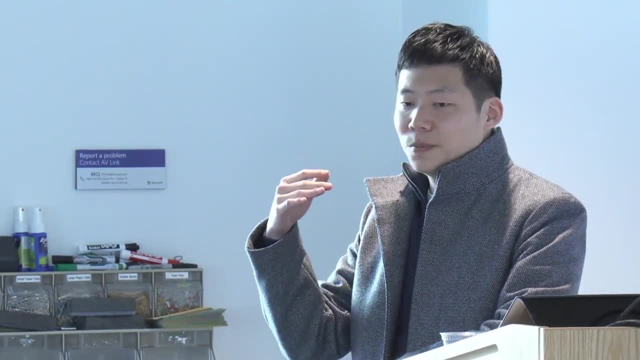 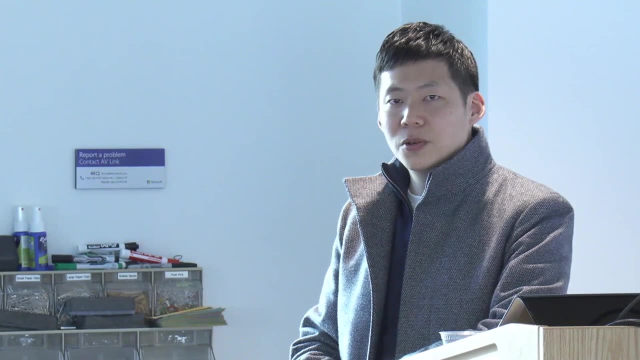 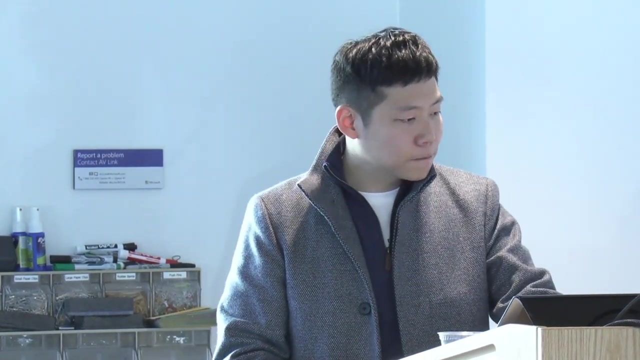 So it is important to manage the scale of intermediate failures as small as possible, not to have this overflow. And another question on the intermediate primes Q1 to QL. So you set them to be equal to the size of the initial scale, right? 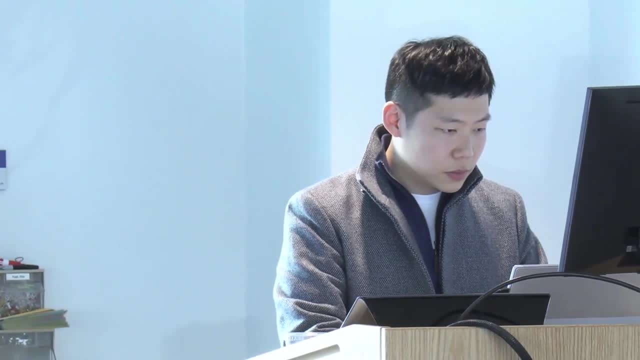 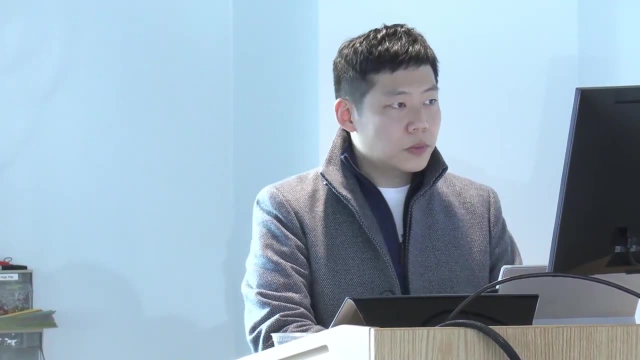 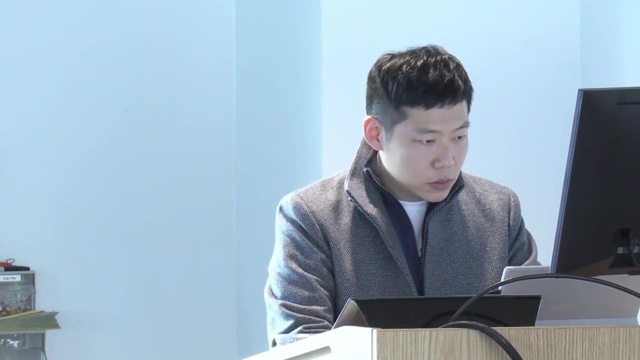 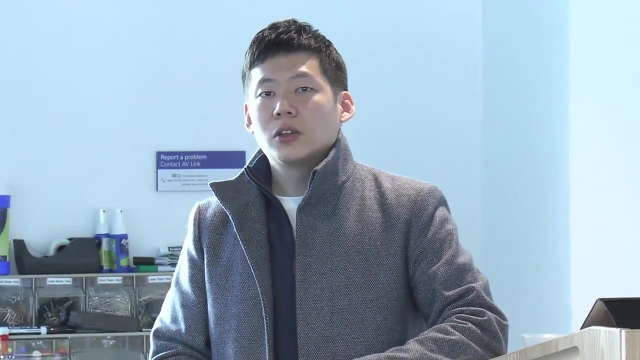 Mm-hm. Approximately Yeah. Is that the best option, or could you also set it? Yeah, Okay, In a different way. So, okay, in general, you can set any chain of moduli. So, because we are going to anyway keep. 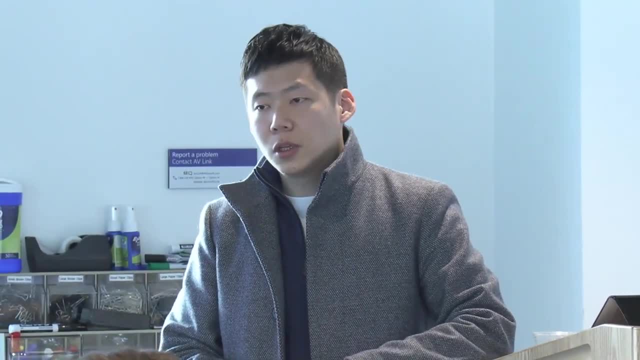 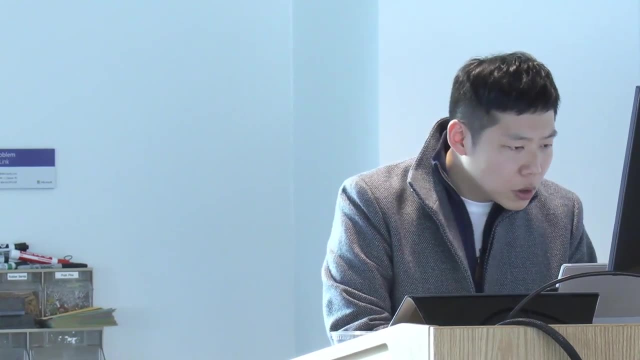 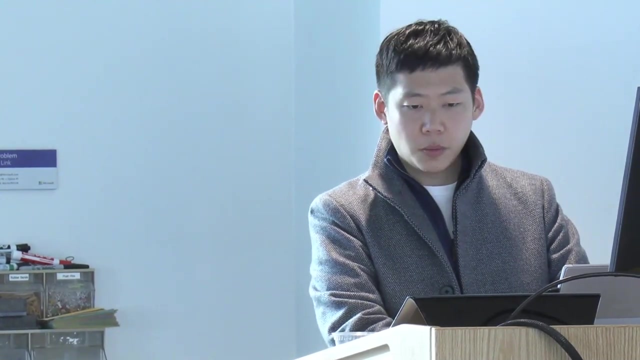 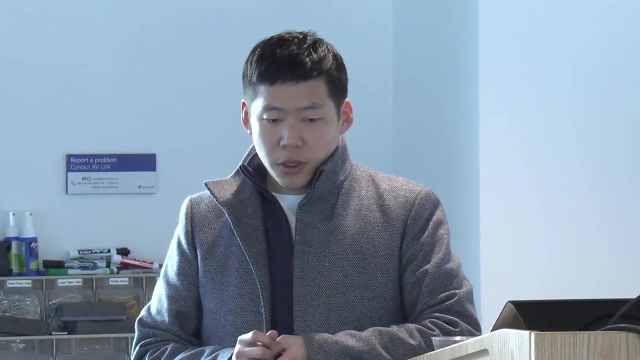 track of the scaling vector following the computation. But the thing is, as you can see, as you could see in this example, over-evaluation of cubic polynomial. Sorry, this is not working. Yeah, So if you want to add some ciphertext with different scales, 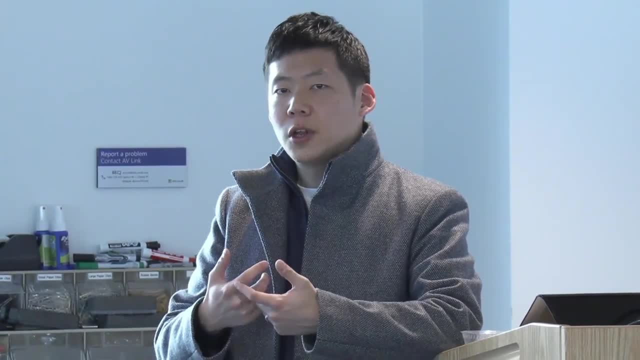 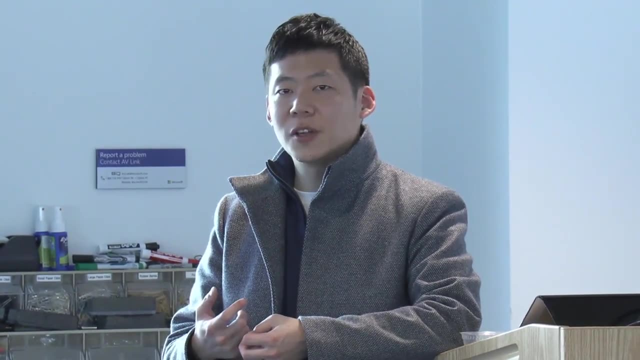 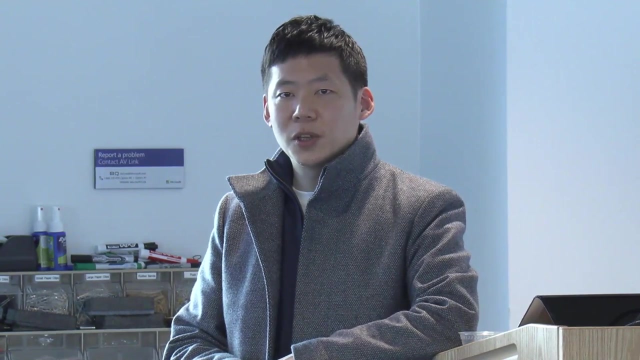 you may consider one level to perform some one-plane cipher multiplication. Let them have the same scaling factor. So we try to avoid this issue and stabilize the scaling factors of ciphertext during computation so that we can just assign, keep almost the same scaling factor data during the computation. 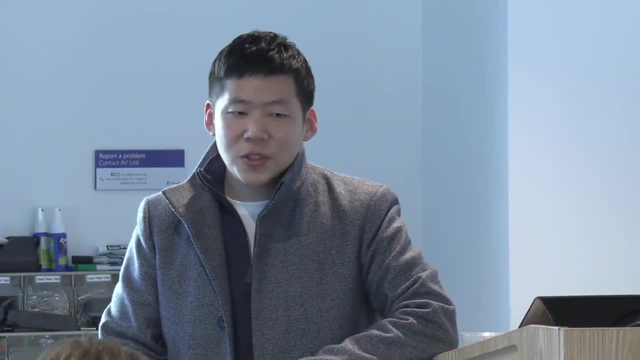 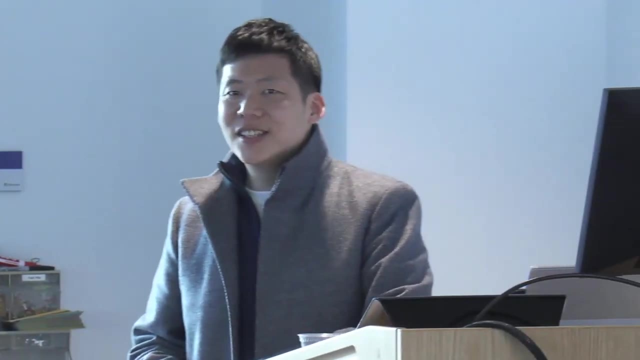 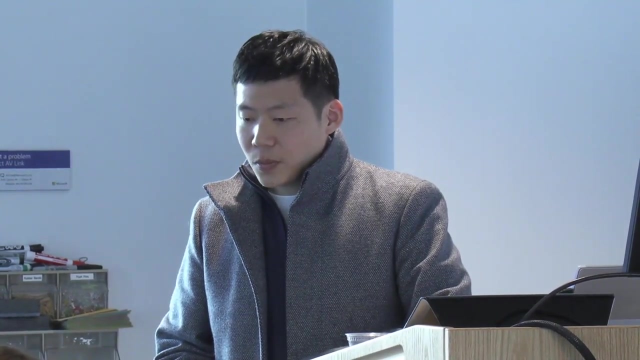 Of course, I'm not sure if there's another, better way of setting parameter, But I would say this is so far the best known method of setting. So in the case of yeah, and there are actually more than one library implementing this,